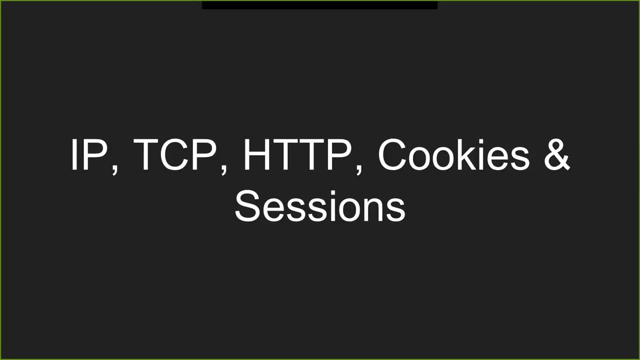 different for every person today. You probably will have seen before, probably know quite a bit about, may or may not know quite a bit about, but this is ultimately going to attempt. It's an attempt to sort of try and fill in gaps of knowledge wherever that's possible. 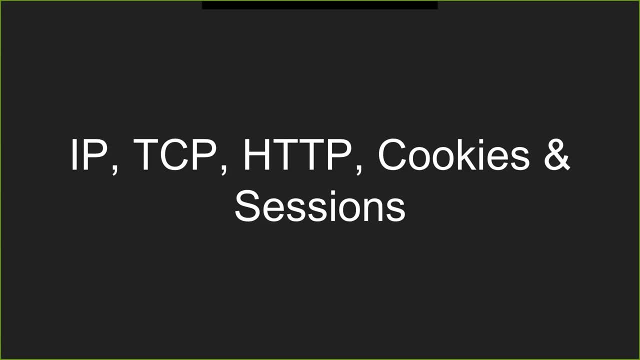 So we're not going to be focusing on particular technology stacks today, We're not going to be thinking even about Node, let alone of like various like servers and stuff and React or anything like that. That's all, not for this lecture, It's all. 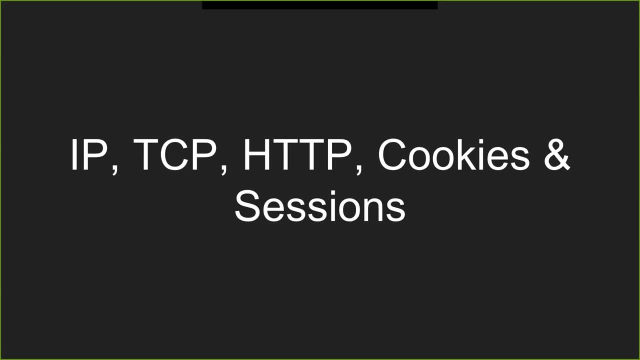 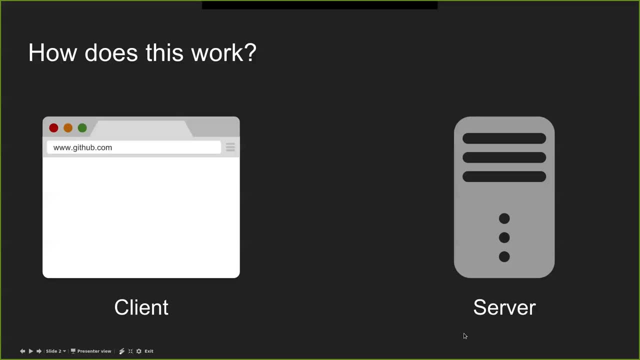 about protocols and theory and stuff like that. So yeah, let's start. All right, so the basic high level thing we're going to be focusing on is a web browser, one interview web page that sends a request to a server, it gets a response and then it displays it. 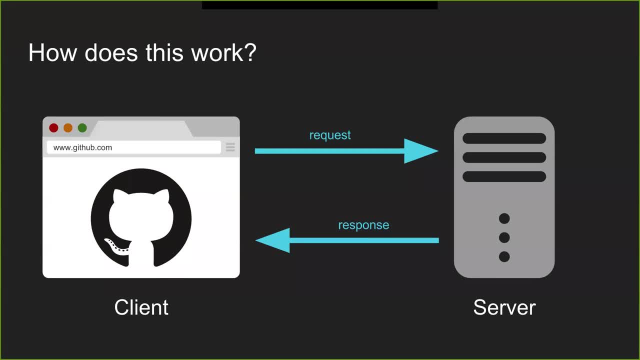 I feel it probably understands the request response idea. You get something, you ask for something, you get it back and you normally focus on two different devices, But there's a lot of things going on here behind the scenes in a very short space of time that we're going to dive. 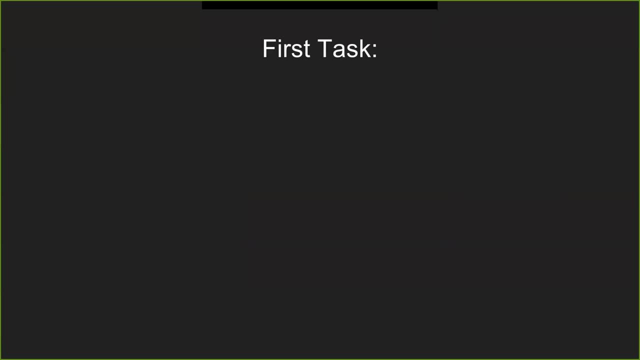 into. So, firstly, what do we need as a first component to be able to do something like this? And that would be: we want devices to be able to communicate with one another. So say, I have a device in one country and I've got a web browser in another country and I want. 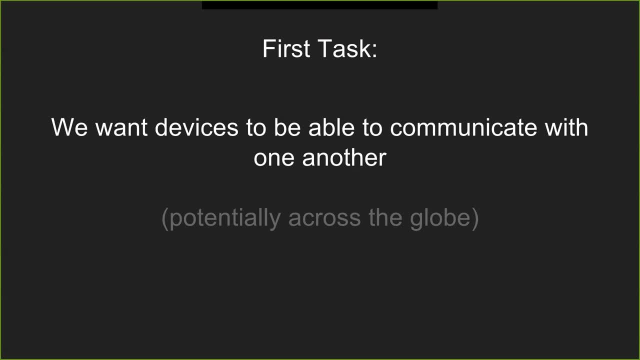 to connect to it. What does it actually mean to connect to that device? How does that work? How do we send the request? How do we get it back? So this is done by something called the Internet Protocol, which you probably have heard of. It's used in lots of 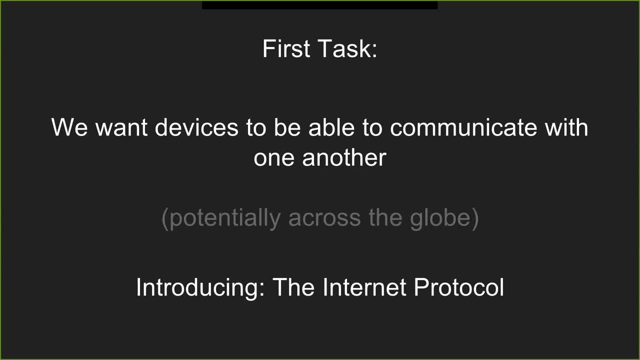 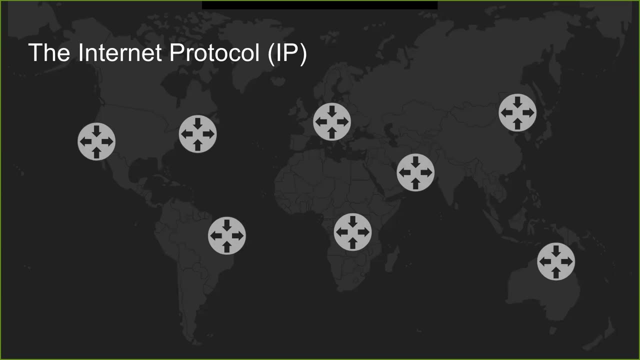 you know common vernacular, Also called IP, which is where IP come from. So what is the Internet Protocol? Basic idea is: if you have a lot of devices scattered around, we're going to call these routers. any device can effectively be a router. 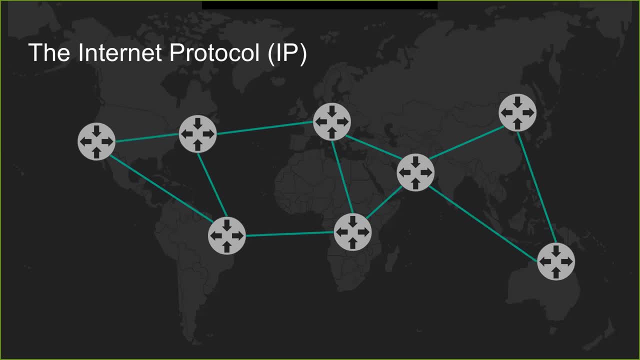 And you have various links between devices. What you want is an ability to sort of send a message message from a device that's somewhere on this network to somewhere else, as long as there's like a path to get to it, and so what we do is we assign each 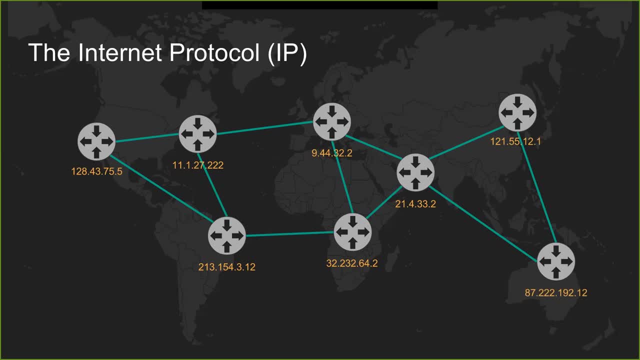 device a number called an IP address. how they get this IP address, I'm gonna, for the time being, go into those details later on. the important thing is, like each device has a unique IP address, that it knows what it is and the things that's connected to know about it and and with that we can then think about. 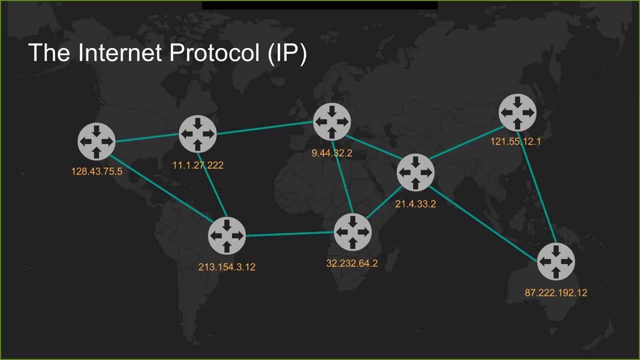 getting. so, let's say, these two devices here and want to get a message from one on the left, oklan, all the way to the one over in Australia. so what happens is constructs, constructs, data, and basically it has information about where it's from, which is its own. 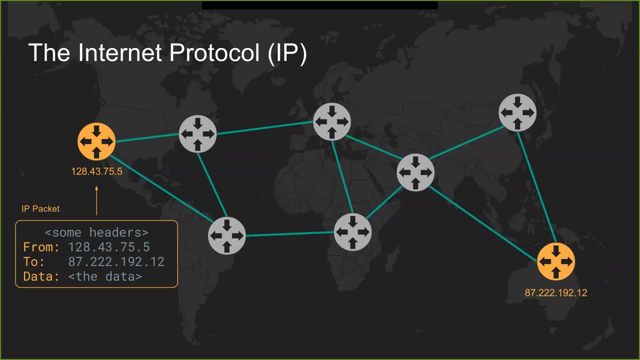 IP address. it says where it's trying to get the message to and then it has like a data that's actually trying to send to the device. by the way, if there's anything that's unclear, if I'm going too fast, going too slowly, if you have any, 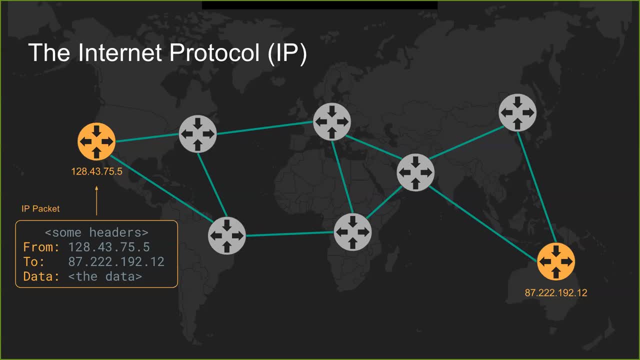 questions. just feel free to like, interject, raise your hand, whatever I want. I do want this to be like interactive as far as talking to you guys goes, but it's not going to be interactive with code. so if you have any questions, let me know. so the device I want to send a message to another device. 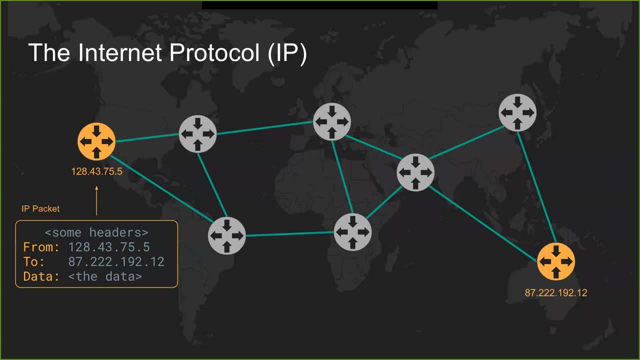 constructs this packet with the IP address is from, the IP address is trying to get the message to and the data is trying to send, and then it just makes a best guess about which router or which device is connected to that it thinks has the best chance of getting that message to where it's intended to get to. 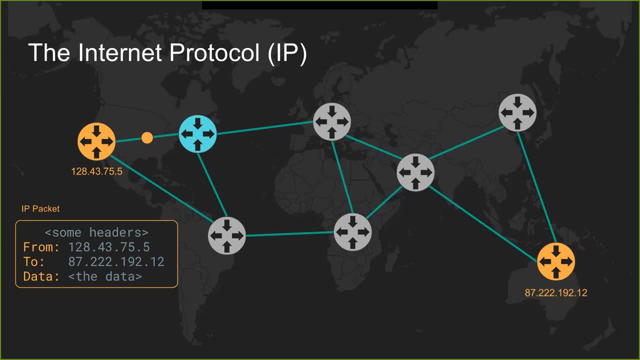 you. so in this example it picks this router. that router then has a look and thinks: hmm, I think if I send it to this router it has a good chance of getting there, so it'll send it to that one. and that router looks like: hmm, I think this router is the. 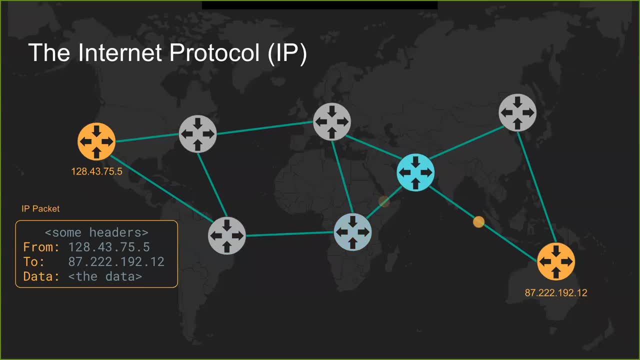 best chance of getting the message to that one, and so on and so on until it finally hopefully reaches the end. yes, right, right. so, um, the question was: how does the router know which one to send it to? how does it make a guess which router wants to send it to? so, uh, thinking about it from like a really, uh, grand scale, 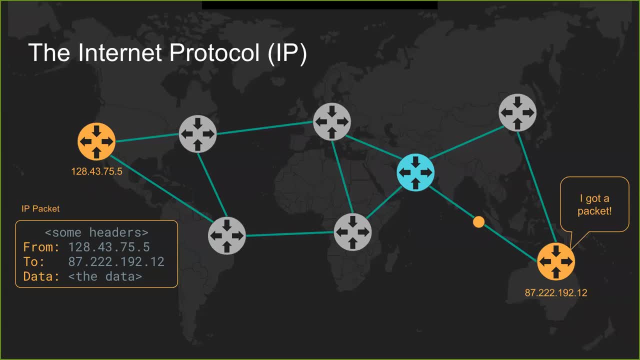 point of view. so, like for thinking like the, the main readers of countries together, I think from a large point of view, each router has a table where it has like blocks of IP addresses that says, okay, these ones belong to this country, these ones belong to this one, and then most likely in that direction and the most 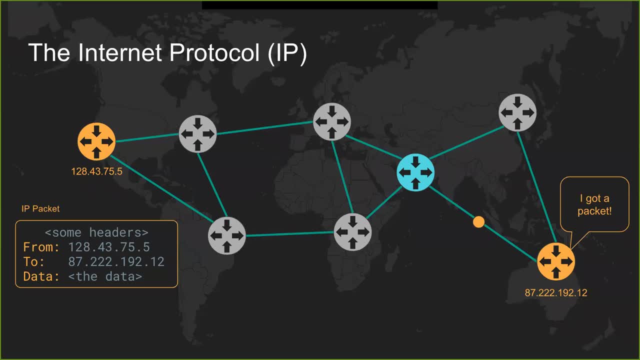 likely connected to this router and the. the short answer is: there's a lot of manual work that goes into that and and there's a protocol called border gateway protocol, which is what you have. so all the internet service providers that are based in all these different countries that have these huge optical fiber. 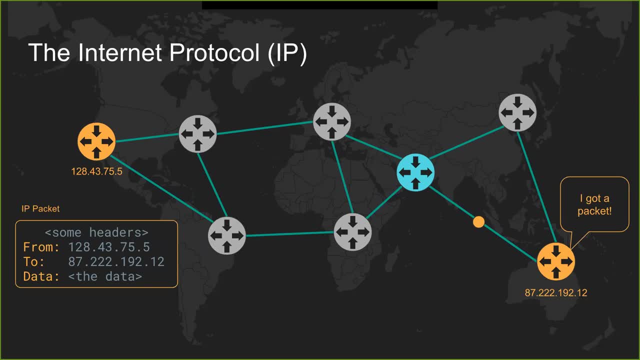 networks and you have optical fibers that going, you know, under the ocean that connect the countries together. these huge, huge data centers are constantly communicating with each other and they're constantly saying, hey, I'm this country and I have these IP addresses. and if, say, somewhere in the Middle East, 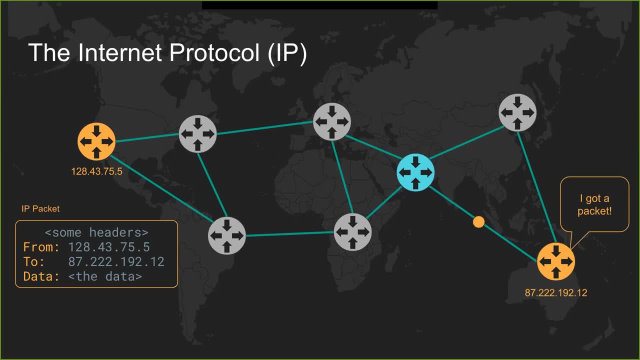 you know in the United States, you know in the United States, you know in the Middle East- sends a message out saying: I have the, I have these IP addresses on my network and it sends out to their countries next to it. those countries will see that and be like: okay, I think I can send messages to these IP addresses. 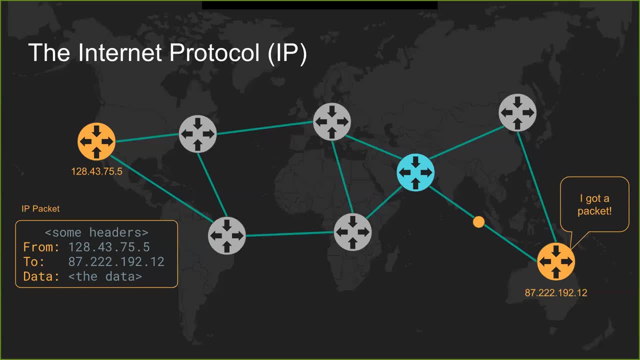 in this direction and but it's ultimately up to those. things like these messages are broadcast and it's up to each individual router whether or not it trusts that message. so there was actually an incident a few years ago. I can't remember the exact details, but it's a country in the Middle East claimed to own IP addresses that Google. 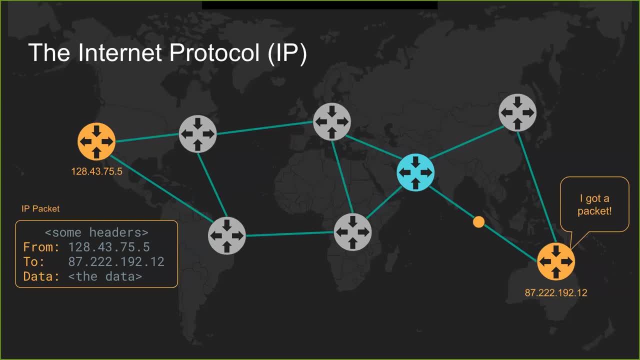 owned and broadcast that message, and for a brief period, a number of countries are routing traffic that was intended to go to Google to these servers in the Middle East. so what Google then did is claimed they sent a broadcast message claiming they owned smaller groups of IP addresses. which takes precedence? which ultimately 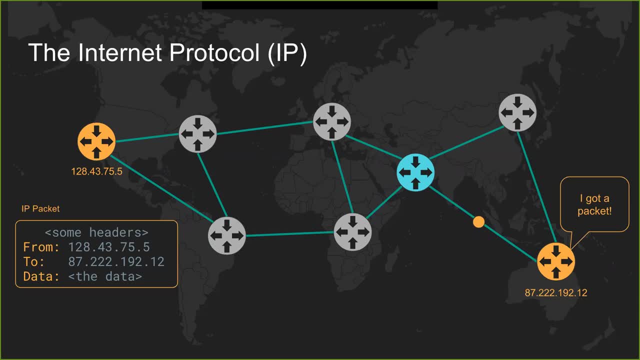 fixed the problem and then temporarily fixed problem until they were able to address the security issue on the world wider scale. so another way of putting it is gossip. that's how these routers know where to send the packets. they sort of just like talk to each other and try. 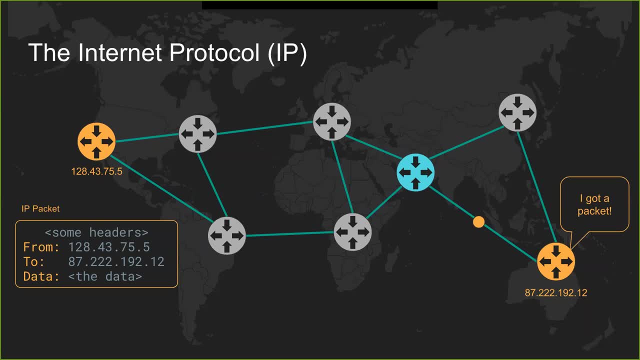 and work it out. that's on a large scale and that figuring it out. that is part of the IP protocol, it's part of the border gateway protocol. yeah, thinking about it on a smaller scale. so if we're thinking about just the like learners guild network, for example, you have, you'll have a router or router. 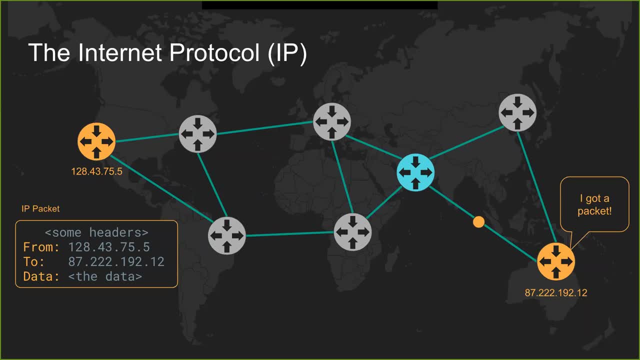 falling into American accents here. you'll have a router or router in the in the building which, when you connect to, will allocate IP addresses. so it says I'm in charge of these IP addresses. actually, I'm just going to go to the next slide, because that has all the details there. 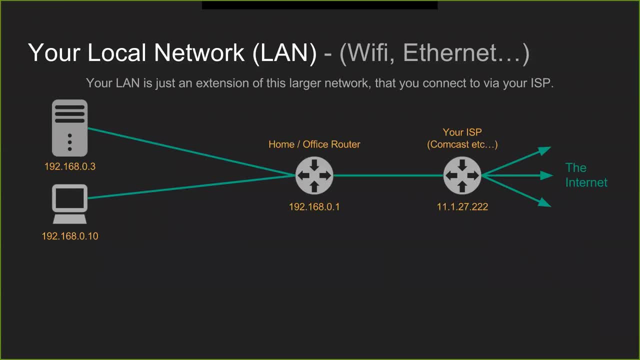 so a local network here, for example, say it's just like an extension of this larger network, so you have all these countries that have all these routers and then that each router there will be connected to like a number of cities and those cities will connect to like routers in like all the small towns and 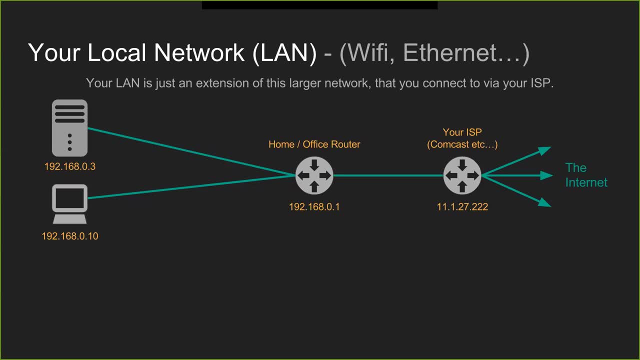 then those small towns will like connect to, like you'll have exchanges and they'll have like connections to each of the homes and in each house you have, you have your own router which then connects to devices in your home. yeah, like a web, yeah, a series of tubes. so it's a. it's very scalable, because if 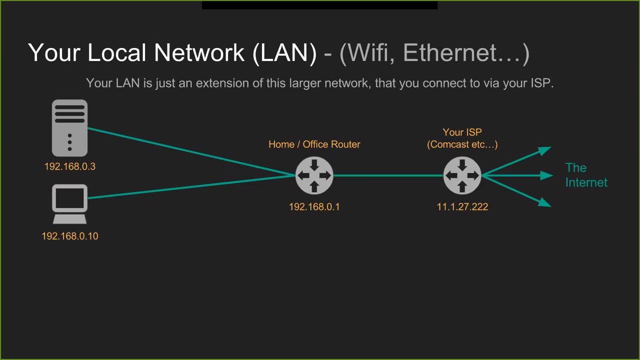 you're, if you just care about like country level connections, you don't need to care about anything below- like the countries you're connecting to and like the major routers in your country, and then each of those routers only cares about like connections in their locality, and then that locality might be like a. 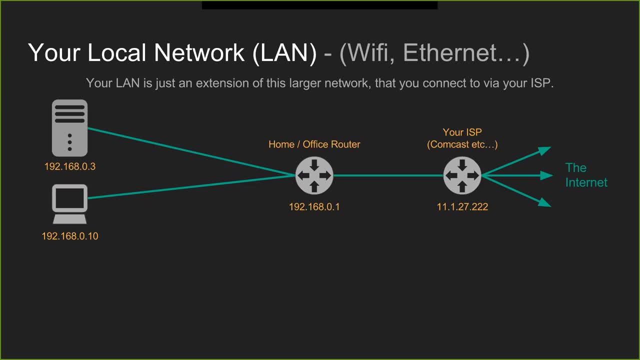 state or a couple of states, and then in there have like routers that might care about just a few towns or a city or only a like a subject, so, and then you get to so like I'm gonna listen so people can see, so this is this ISP, here this router might be connected to like thousands, or 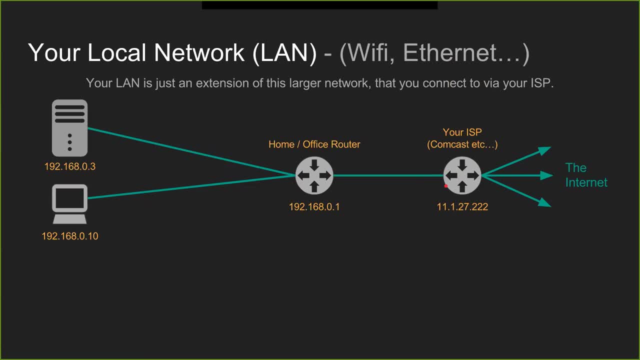 tens of thousands of homes in a particular city, and each, each house, has a connection to app, and this router here is in charge of the devices in your home, and it will. every time a device connects to it, it will allocate a new IP address that it has control over, and so this route in those more accurately exactly. 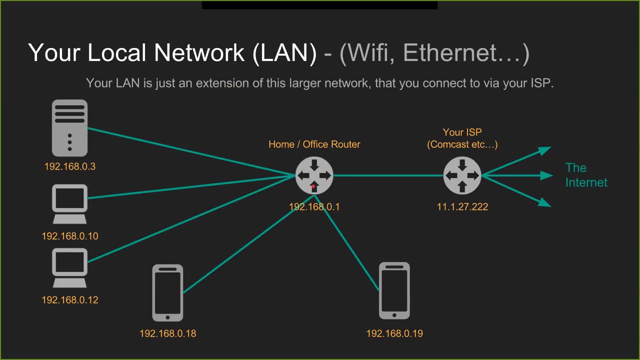 where the IP addresses are a question. so if an infrastructure is running on a certain type of network, you need to know exactly how many devices are connected to it. so if an If an IP address falls within the range that it controls, it can send it directly that message. 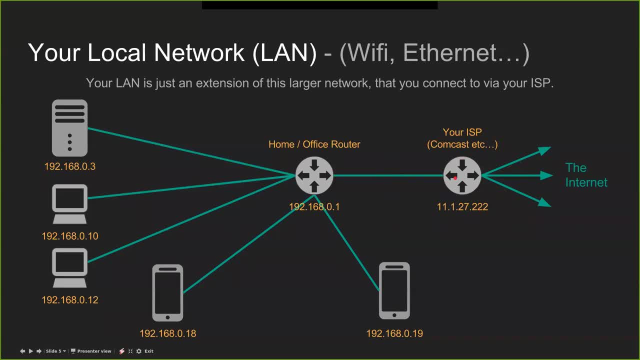 If it isn't one of those IP addresses, this guy knows where to send it And it's pretty simple. It's either on my network, and I send it directly to the device on my network, or it's not on my network. 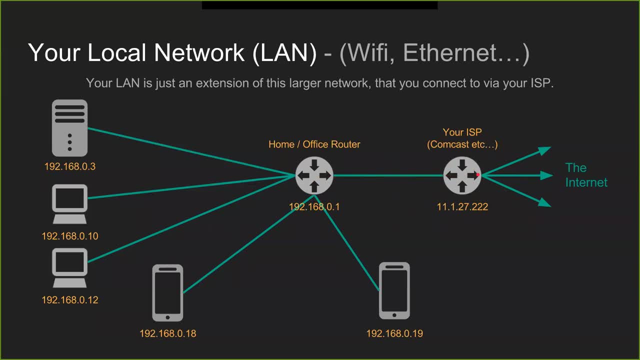 and I send it upstream And that's sort of the general structure that you have until you sort of think about things on a country level where it uses BGP- Cool, Can you say the name of that? border Border Gateway Protocol? Yeah, 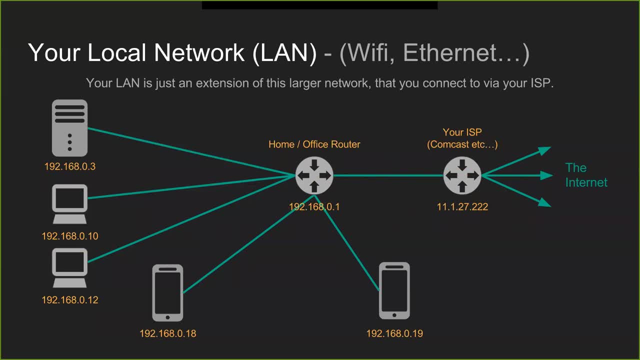 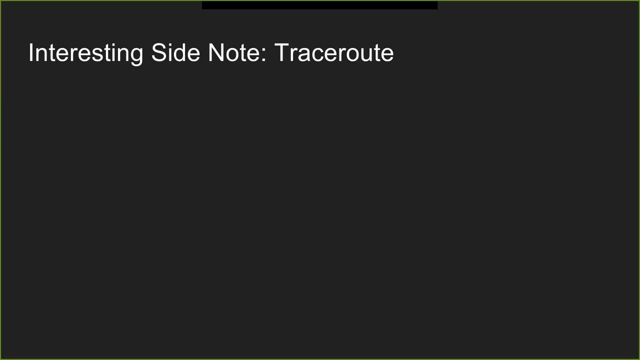 I think, Border Gateway. Let me just confirm. Yeah, Cool. Any questions for anyone from this? All right, So there's this cool tool called Traceroute that's available on most operating systems. that actually allows you to sort of inspect the route that a package will. 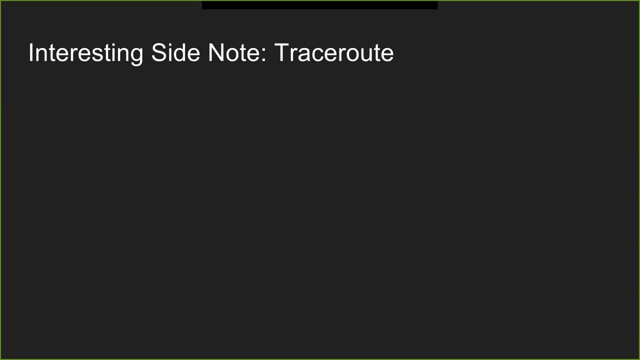 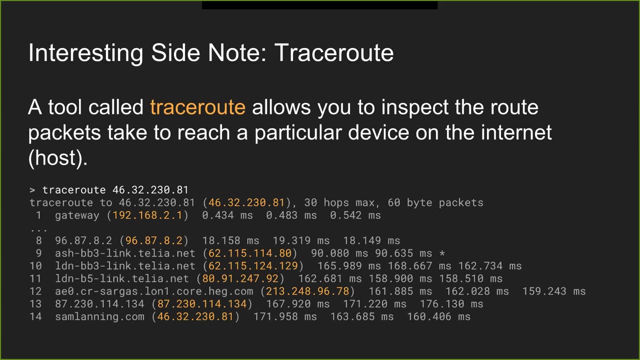 take when you try and reach a certain address from your own device. So here's an example Traceroute from my home to my website. So I'm like, can you tell me what the route is here? And the first hop is: this is my home router. 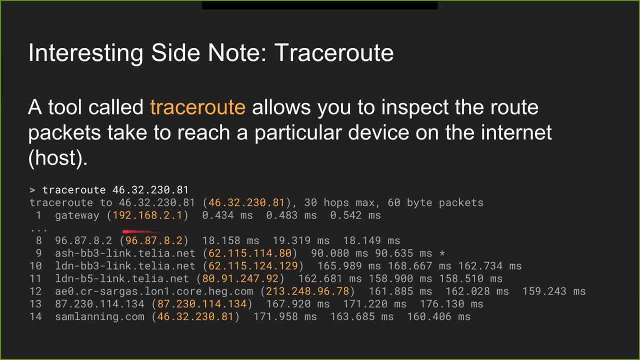 And it goes through some various things Before it's reached the UK and it goes through some routers in the UK until it reaches my ISP and then finally server-based in the UK, And each of these things here is a different router. 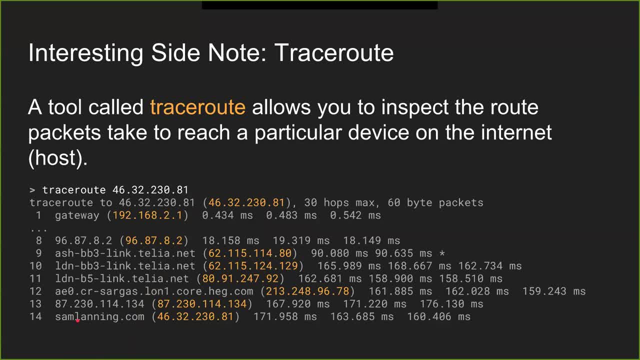 So it has like 14 hops to finally reach my server. I might go into details about how this works later on, if there's time, but it's not too important, All right. So if we think about our end goal again, it's just you know. 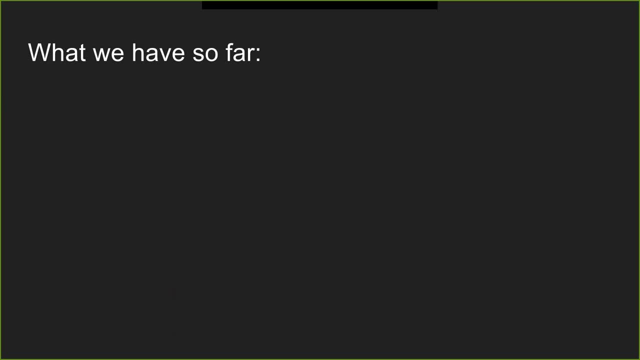 our end goal. again, we're trying to get a web browser to be able to view web pages. So send a request, get a response. So what are the components that we've described so far? So we have a way of identifying devices. 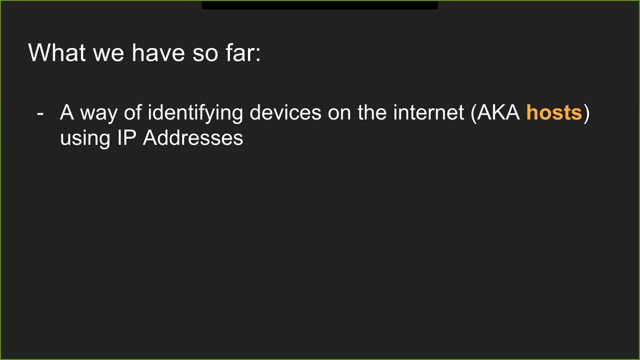 on the internet, which we're going to call hosts, using IP addresses And we have a way of sending small packets of data, like in the general direction of the devices we're trying to communicate with. Is this enough technology? Is this enough technology that we've 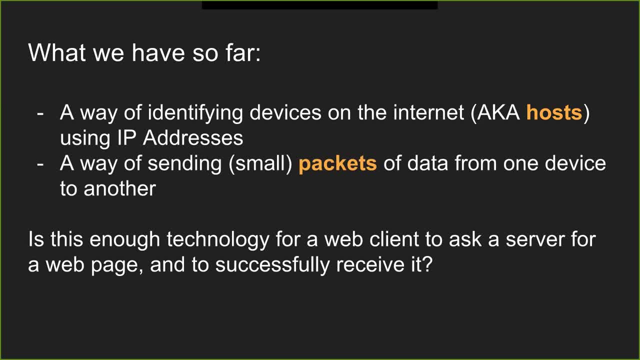 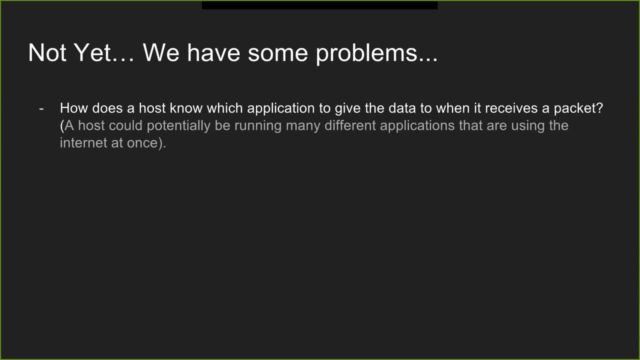 introduced to be able to display web pages on a web browser. Not quite yet. We're missing a few things and we have some problems. All right, So if you have a host device, it could potentially be running many different applications, Like you might have a web server. You might have some other servers doing other things. You might have a chat server. How does the device know, when it receives a packet from someone, which of those applications to give that data to, especially if they're all trying to use the internet at the same time? 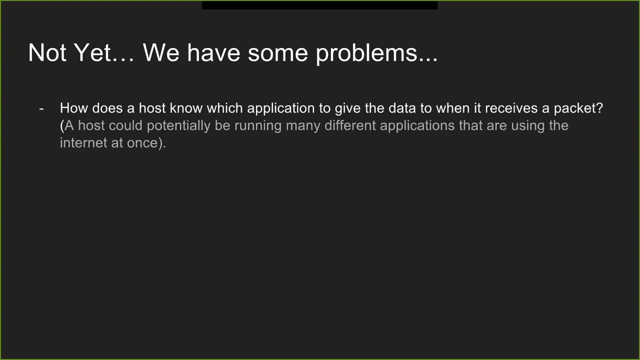 That's not something we've addressed yet. We just know how to send something to a device. We don't know how to send something to a specific application on a device. Another problem is that packet delivery over the internet is unreliable: Packets could get dropped, corrupted, duplicated. 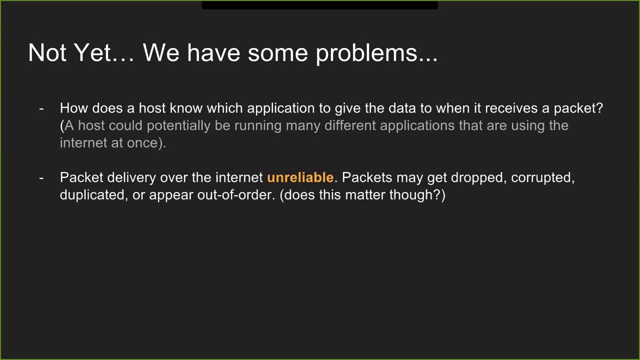 You could receive them out of order And there are many different reasons for this. It's not guaranteed that the packet's going to take the same route every time you send something to a server. It might go one route another time. It might go another route another time. deal with congestion If routers come online offline. the shape of the internet's constantly changing, So there are lots of reasons why packets may or may not get to their destination- corrupted, duplicated, out of order, et cetera. So this is something we need to account for. 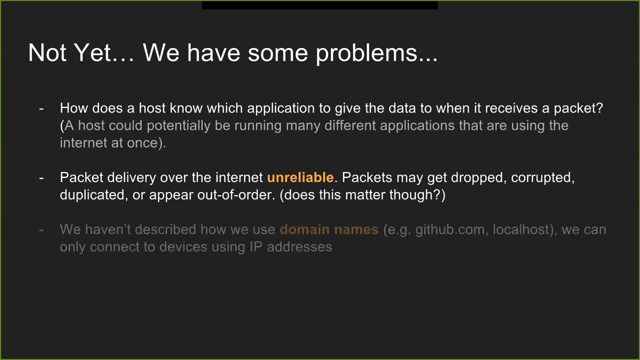 when we're trying to send data from one device to another, And there are a couple of other problems. We haven't yet described how we get from domain names to IP addresses like githubcom- to what's the IP address of the server that's hosting githubcom. 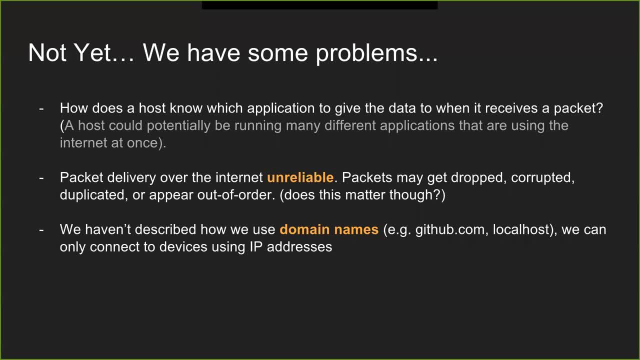 We don't have that information yet, We don't know how to get that information, And we also haven't described what a request from a computer to a server looks like when we're trying to get a web page. So what does the client send to the server when it's like 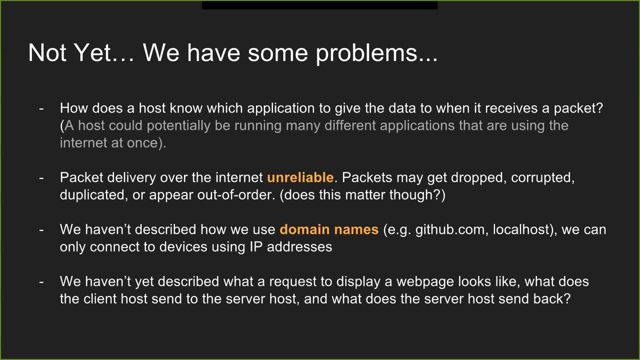 I want to view this web page, And what information does the client, does the server, send back? So let's deal with these two problems first. So we want to be able to direct messages to a specific application on a computer, not just the computer itself. 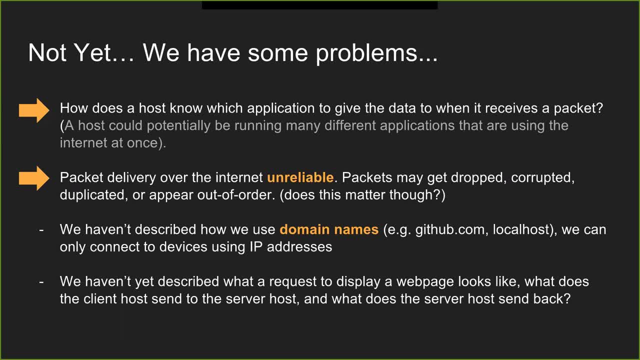 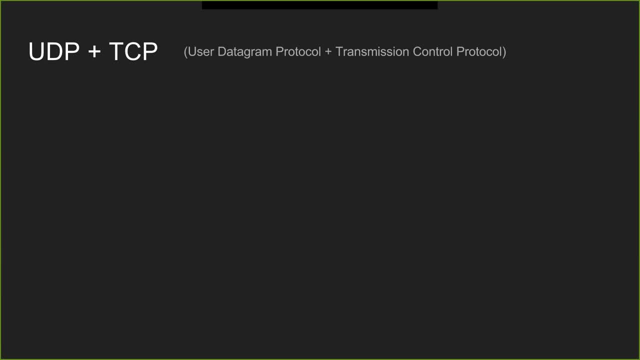 And we want to make delivery of packets reliable, So we're going to introduce two protocols called UDP and TCP. Has anyone heard of these before You've heard of TCP? Cool, All right. Does anyone have what we think is a basic understanding? 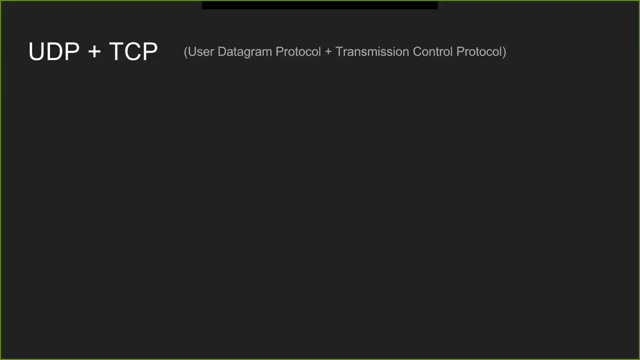 of what these are? Cool, All right, Nice, fresh start. So these are two protocols that are built on top of the internet protocol. They're actually part of the internet protocol suite And they were all released and made like a standard at the same time. 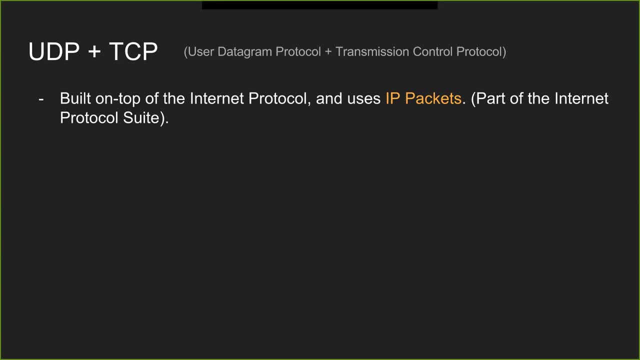 And they, Yeah, Send their data inside of IP packets, And it allows for many different applications to receive data on the same host by listening to different ports. Who's heard of ports before? Yes, cool, 3,000,, 8080,, whatever you fancy. 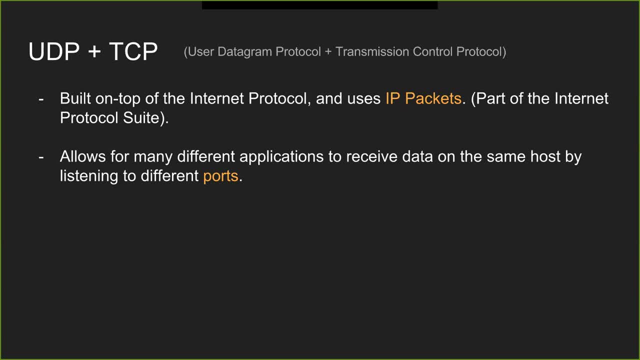 Yeah, So ports are something that you can see in the URL And that's just using the default port. Does anyone know what the default port for HTTP is? Nope, No, 3,000.. Nope, Nope, All right Cool. 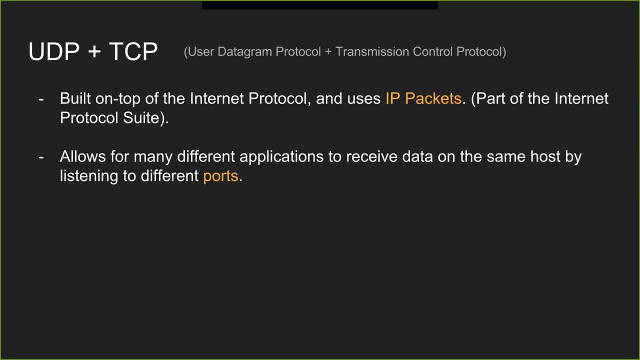 This is great. I get to introduce more information. We'll come to that in a later slide, So I'm actually not going to tell you what it is now. I'll leave you hanging. Cool, So UDP and TCP aim to Yeah. 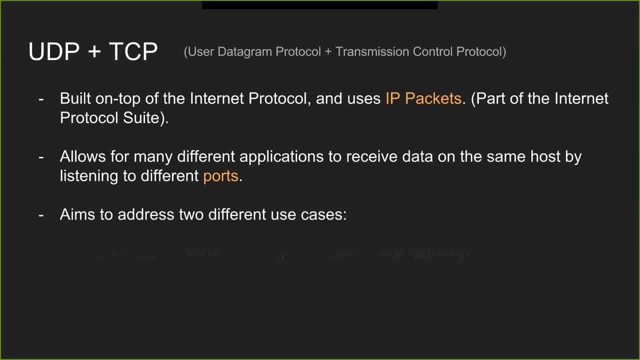 Be optimal for two different situations. So UDP is useful for applications that require low latency. So they are optimized for things like video calling, voice calling, multiplayer gaming, streaming. UDP is not a reliable protocol. It just aims at getting the packets to a specific application. 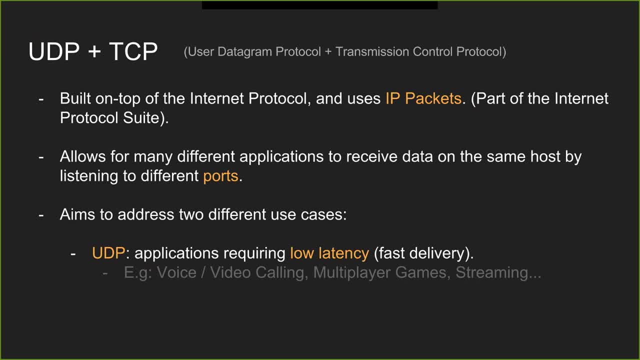 It may or may not get there, It may get corrupted. So it still has a lot of the same problems that sending raw IP packets has- Wow Cool. The other use case, TCP, aims to give reliable delivery of information to a device. 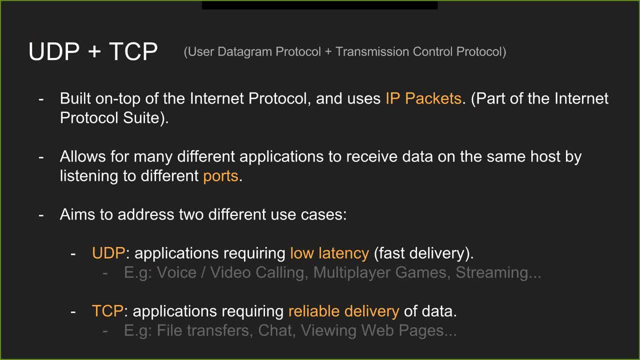 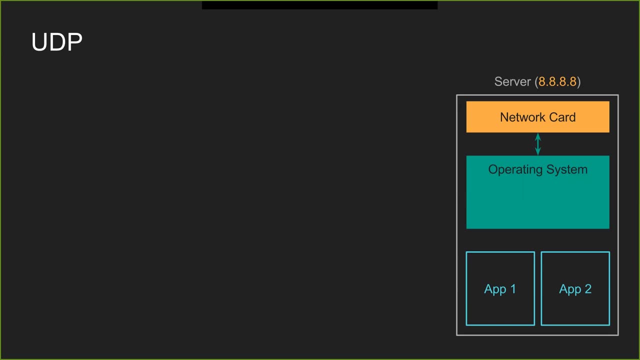 So I think using that for file transfers, text chat and viewing web pages, which is ultimately our end goal with this lecture, Cool. So how does UDP work? So thinking about it from the server side, a server that wants to be able to receive information? 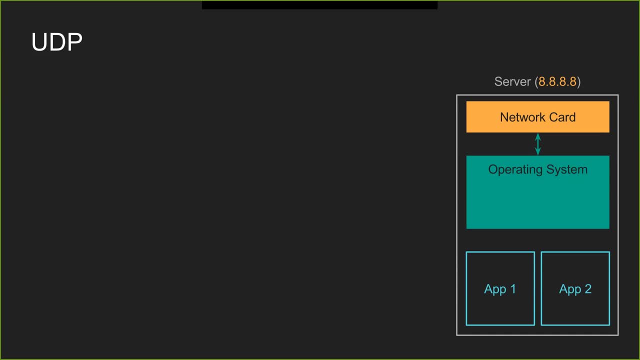 from a device. Yeah, Yeah, Yeah, Yeah. So let's say we have two applications on the server. I'm just going to switch. That's why I can't do it, because I've still got the pointer mode. OK, So the application first requests hey. 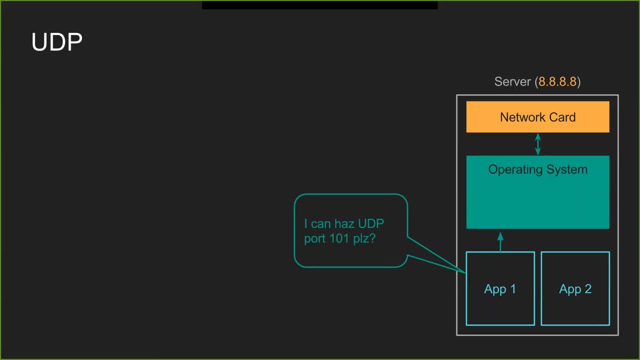 can I receive all the UDP packets that are addressed to this port. So it says, can I have port 101?? And the operating system then makes a decision whether or not to allow that And it says, yeah, Yeah, sure, Go ahead. 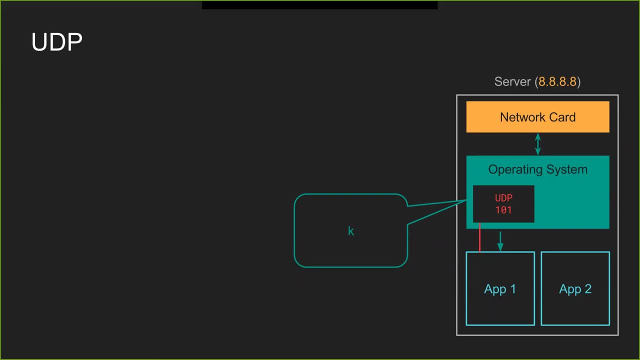 So application one will now receive all UDP packets that reach this server that have port 101. And say: application two then is like: hey, I also want to listen to port 101. The server will reject that because port 101 is already assigned to an application. that's listening. 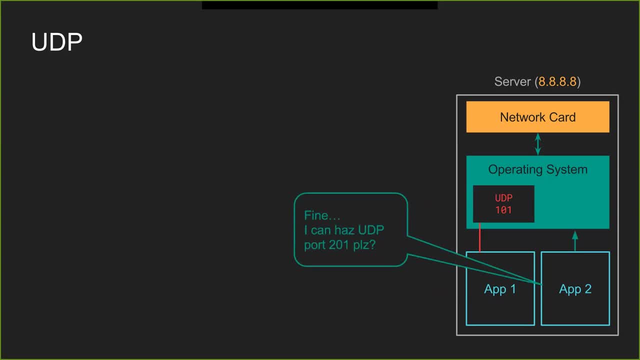 The application can then be like: can I have port 201? then Yeah, Yeah, Yeah, And then, yeah, the operating system might grant that request. So now we have a server that will accept packets for two different UDP ports and forward them. 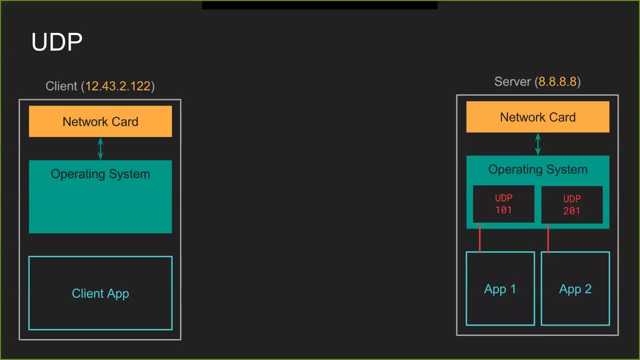 onto the right application. So now, if we bring a client into the picture, a client that wants to send UDP packets to the server, firstly the client's- oh, I don't know if they're connected over here, Maybe the internet, of course, because that's necessary. 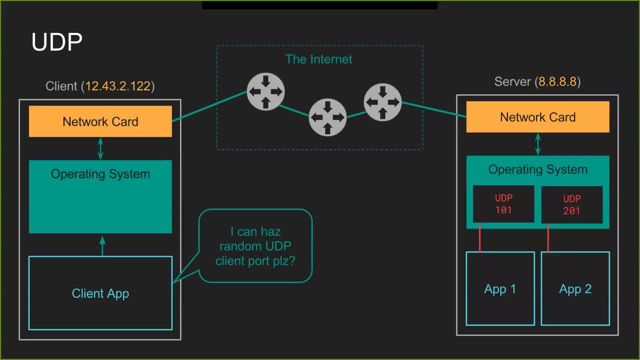 The client says: can I have a random UDP port? I don't really care what it is, but I need a port to be able to receive my responses. So the operating system will say you can have this port to receive responses on. 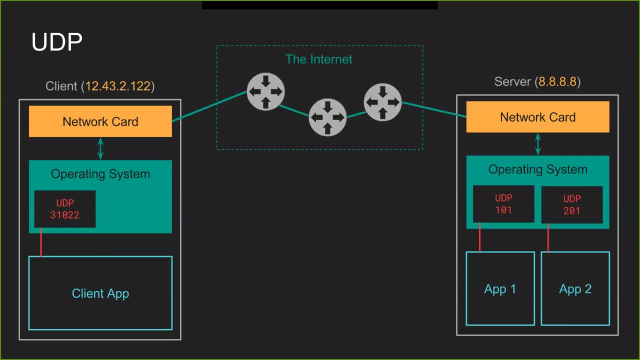 and then assign a port to it, And then the client can then construct an IP packet which has- and this is so- IP. IP also allows you to specify which protocol it is, And then that allows the operating system- and it receives a packet- to know how. 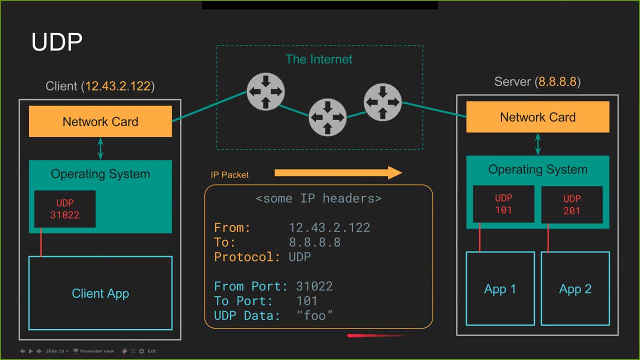 to deal with the data, which, for UDP, is this stuff here? So UDP has a from port and a to port, just like there's a from IP address and a to IP address. So this client app is sending a message from port 31022. 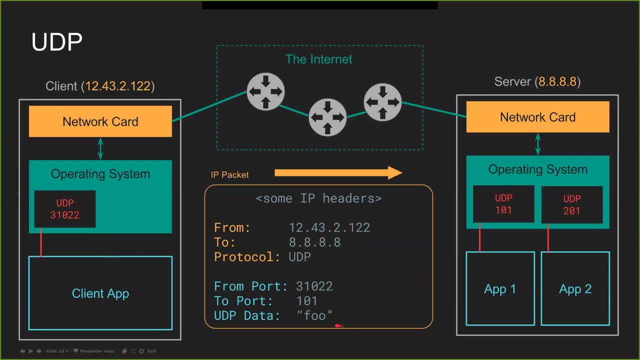 to port 101 to this device here and it's sending this data. So the client sends it to the operating system, which sends it to the network card. The network card will be like cool I know how to set. I think this router will be able to send it. 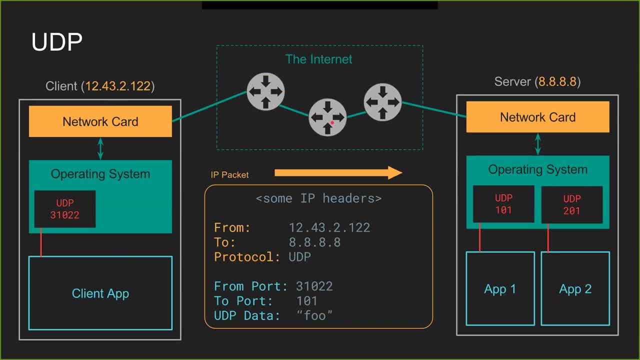 And then this router is like cool. I think this router will be able to send it to this destination, so on and so forth, until it reaches the network card of the server you're trying to reach. And it's like cool, that's me. 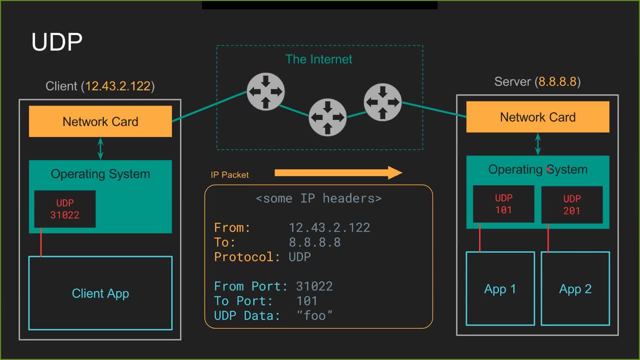 I can deal with that request. And then it sends it on to the operating system. It's like: hey, we've got a UDP packet for 101.. And it's like: cool, I have an application that's listening to that right now. 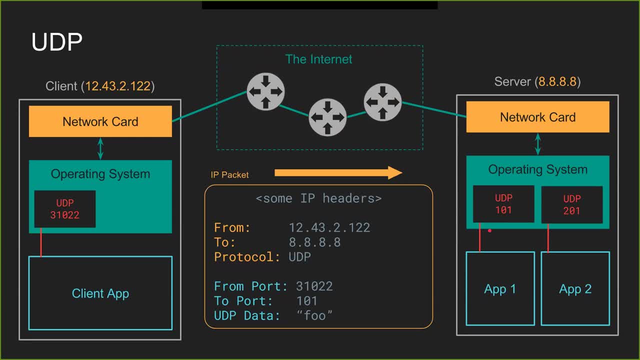 I'll send it on to that application And then application. one gets the packet And then application. one can respond, construct a packet and be like: cool, I'm going to respond with my own UDP packet back to where it came from. So it sets the to port to the client port. 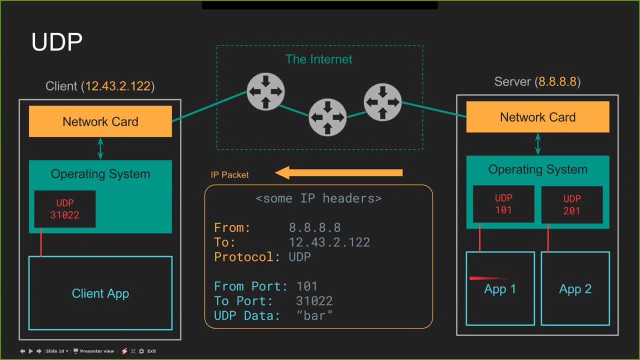 that this client requested sends it on to the operating system, which sends it on to the network card, which sends it over the network card. The network over the internet gets received on the network card, on the client, which passes on to the operating systems. 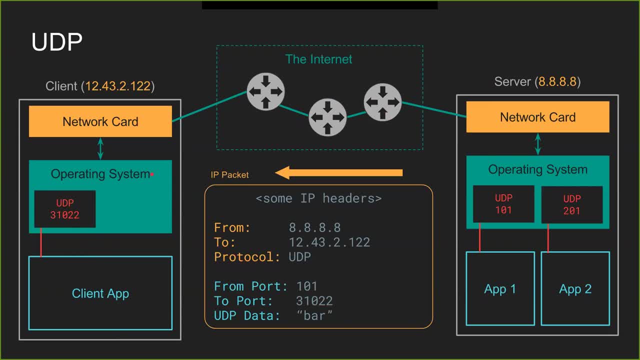 like, hey, is there anything? listening to port 31022 on UDP? And it's like, yeah, there is. So I'll send this message on to the client app And that's basically how UDP works. So you're going to have about 64,000 ports. 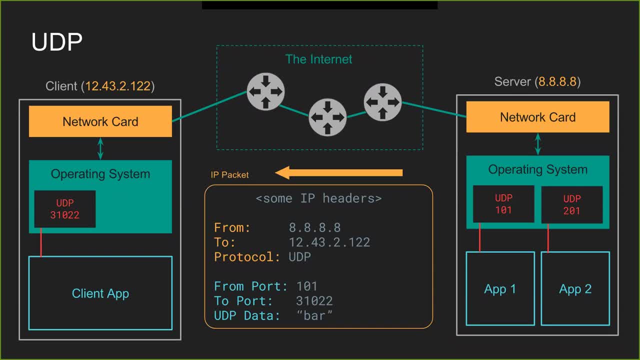 that you can choose from, which is a lot, So you can have many different applications, And applications can listen to multiple ports as well, if they want to. There's no reason why an application is only allowed to listen to one port, And that's how you direct messages. 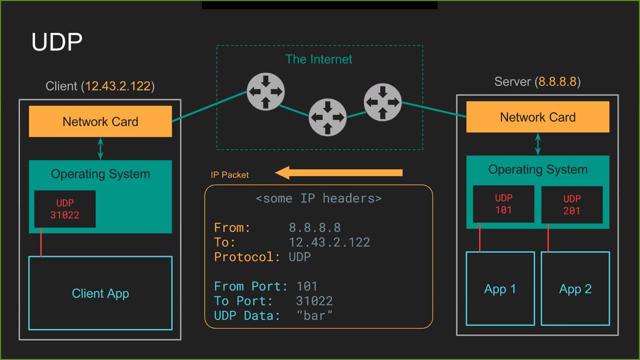 to a specific application on a specific device. Yes, What defines or delineates an application, Like if I'm on Chrome, that's an application And if I'm on googlecom, that's an application? Right, If I'm on googlecom, that's an application. 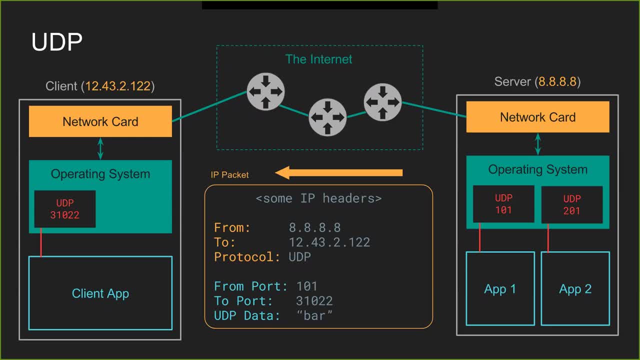 Right, And if I'm also on GitHub, are those two separate ports on my computer technically? But then is it like 31022 or 31023? Right, So it's basically up to Chrome. What it decides is different applications. 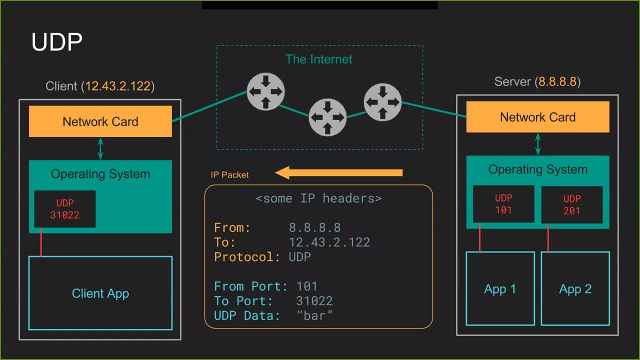 Like, an application can split itself up in many different ways. You can have sub-processors, You can have threads, et cetera. But conceptually, for the purposes of this lecture, Chrome is a single application, A single application which map. 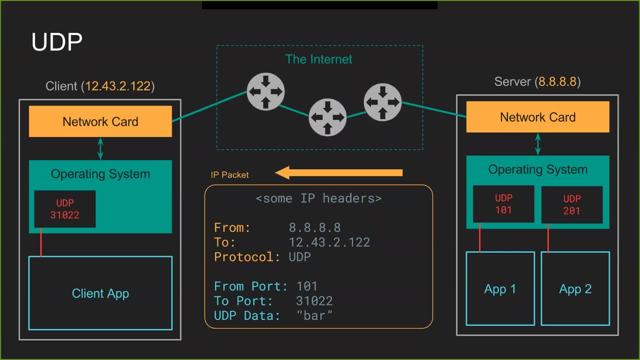 may make many different requests. It might have many different connections open at the same time, So it might decide to ask the operating system for dozens of these ports to receive messages from. If it's on one port, then it has the ability to take the packets that it's getting from GitHub. 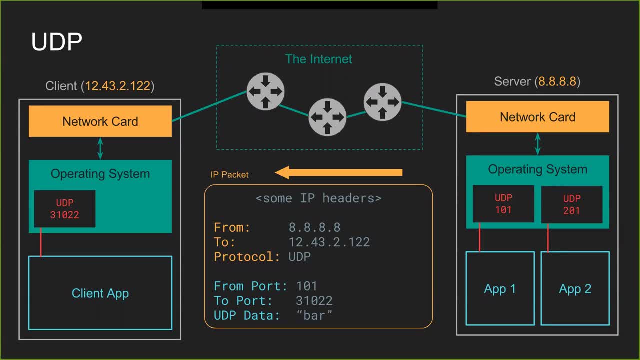 and put them in a different window, then Right, yeah It. then yeah, it can take each packet and be like: OK, this is for this window, This packet is for this window. OK, But there are a few more layers between actually receiving. 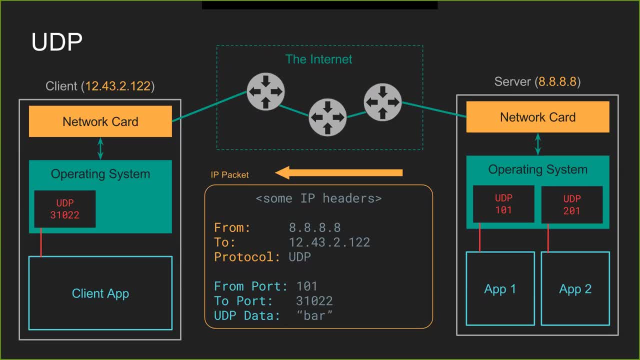 a packet and displaying a web page, which I'll be going through in a bit. But ultimately, yes, if the application is receiving data from many different sources in the same port, it can then make a decision how it's going to use each of those packets individually. 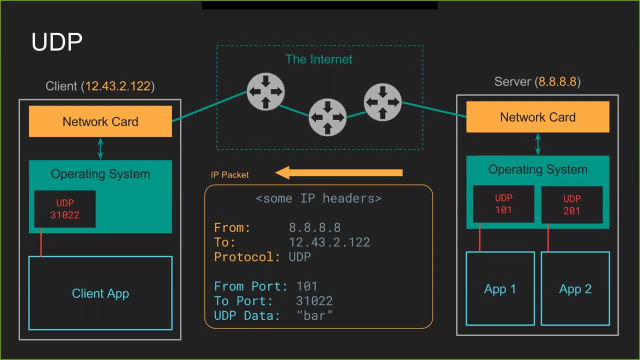 And it might demultiplex them is what it's called. Yeah, This is a lot of information that I've just thrown at you, So don't worry if you can't digest it all immediately. It's being recorded so you can look over the video. 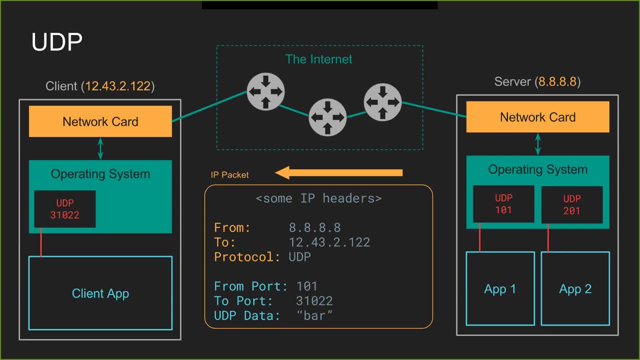 when it's on YouTube. But for now, are there any other questions that people have before I move on? Cool, OK, So that's UDP, That's how you. oh, yeah, It's a network card. Yeah, In your computer you have a network card. 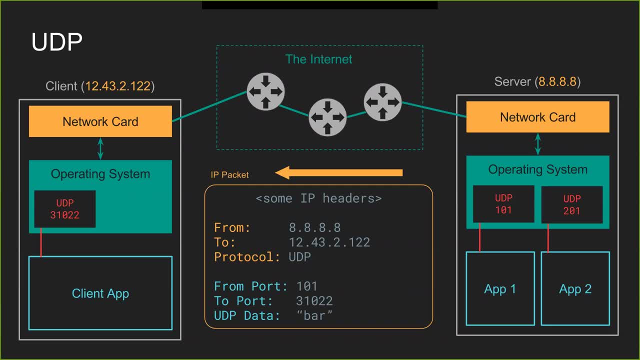 And that just knows about your local network rather, I guess Right. So again, here it's more of a conceptual thing, But yeah, it can be a physical thing. It generally knows it's connected to this network here And it has this IP address. You might have multiple network cards if you connect to Wi-Fi as well as well as Ethernet. Phones are an interesting example, because you might be connected to five or six different networks at the same time over LTE, 4G, Wi-Fi, Bluetooth, whatever. 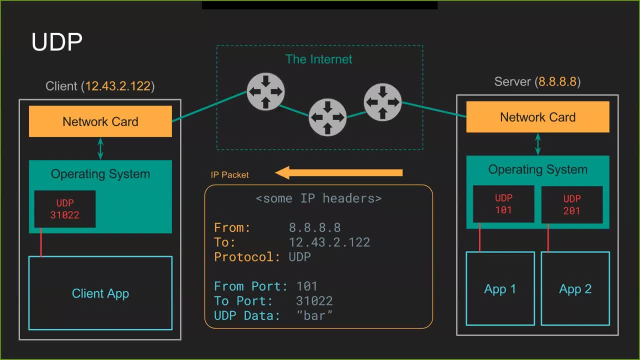 All of these are potential ways in which your device can be connected to the internet. What about a SIM card? So yeah, a SIM card wouldn't be the network card, It just contains information that allows you to use your network card to connect to mobile networks, mobile providers. 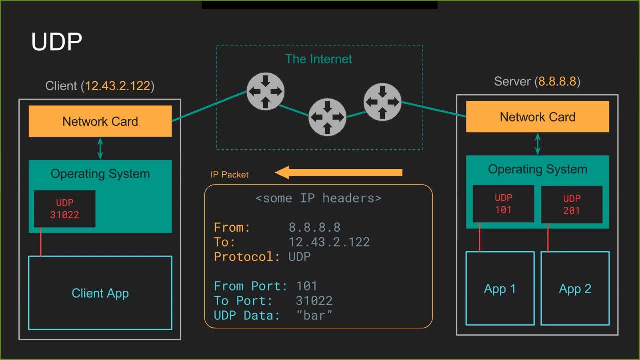 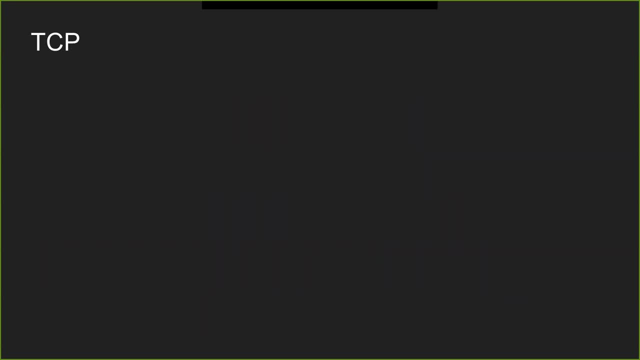 OK, Yeah, Cool, All right, so TCP. So we still haven't solved the problem of data delivery being unreliable and not being able to actually get it all the way to the server. So TCP solves that. It's pretty similar in that it uses client and server ports in the same way. 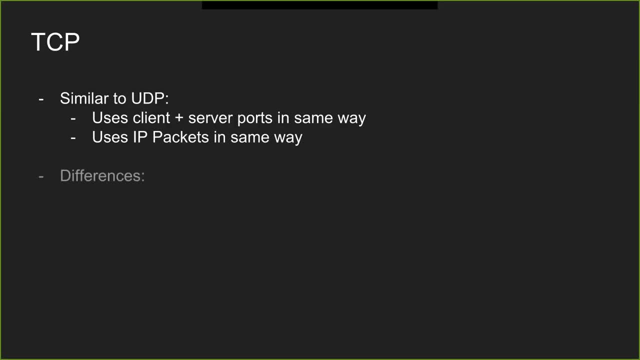 Ports are the same thing. It uses IP packs in the same way. Where it differs is before you can. before an application on one device can send TCP data to an application on another device, a handshake needs to take place. There needs to be a connection established so that both applications know all right. 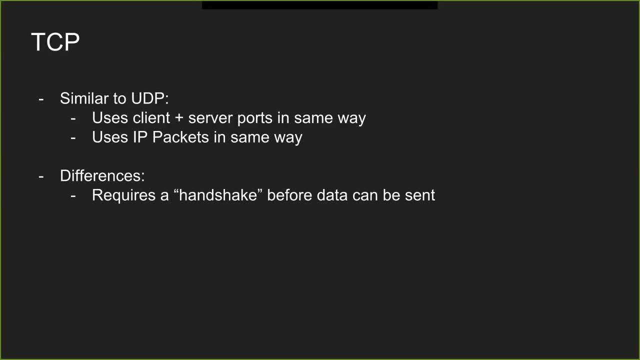 the other application knows I'm trying to send messages to it. It knows I'm connected to it. Let's try sending things. And each packet that gets sent over TCP gets associated with a number, so that missing and corrupted packets can be resent and duplicated packets can be ignored. 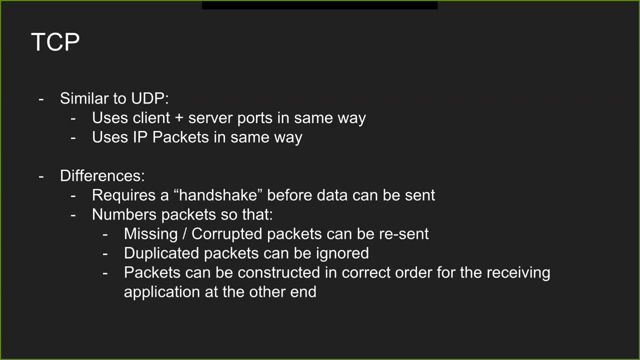 And when you receive all the packets, because you're likely to receive them in the wrong order, you can reorder them so you get them, like if you you know you get them in the right order Or you can read them in the right order. 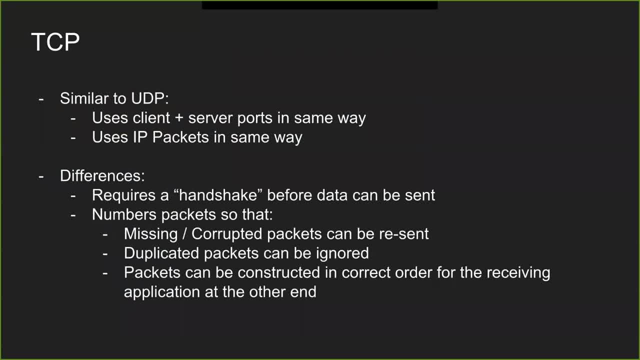 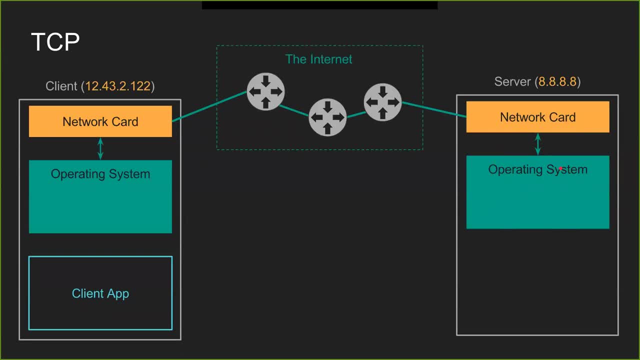 Yes, Is that process when you said if you get it out of order, you can reorder it. how does that happen? So that happens transparently in the operating system before. So as an application, you don't really don't need to worry about that. 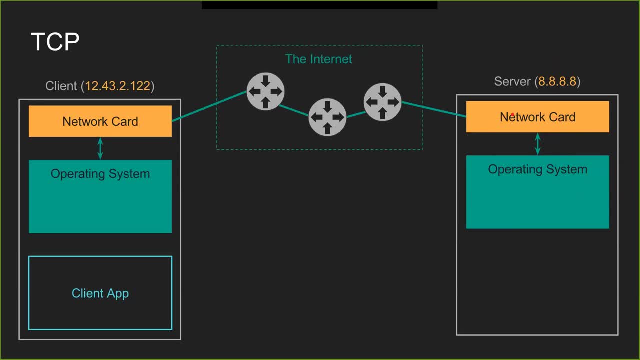 And sometimes even happens in the network card Rather than actually the operating system. it might be on a completely different like chip that actually does this work. So it kind of re-scrambles it. Yeah, it like it, like unscrambles it. 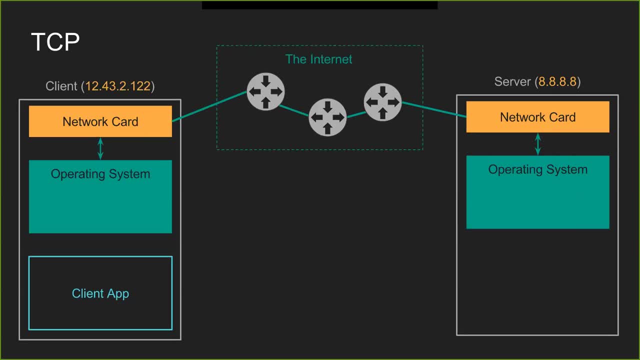 So you have the, so you have an, so, as an application, you never need to worry about, unless you're using UDP and you actually want that behavior and be able to like, like, handle that stuff yourself, Like if you've got video chat and you're just trying to send as much data as possible. 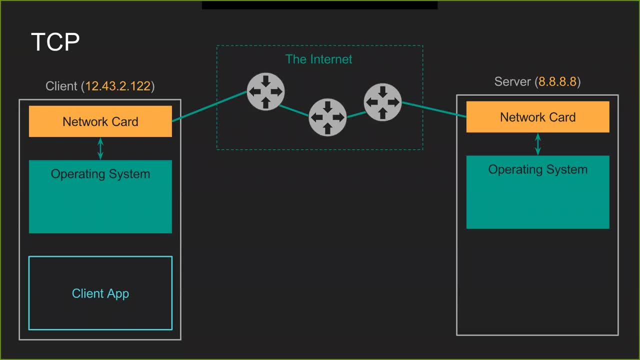 and then make sense of it at the other end. only at that point, as an application, do you need to care about the order In which things come and whether or not packets are corrupted. As far as if you're, if you're an application and you're using TCP, 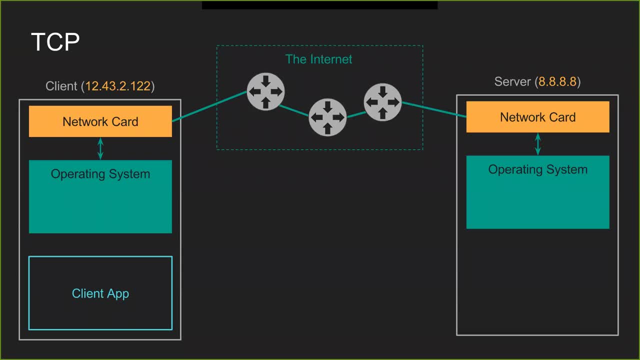 that's all handled. all that data is like unscrambled before you as an application will see it Either in the operating system or in the network card. So the way that TCP works, let's say, if we assume that we have two applications on the server listening to TCP, ports 101 and 201,. 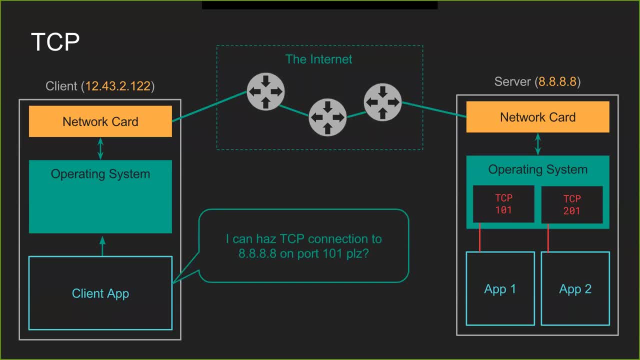 and the client. we have a client app on a client machine that wants to connect to TCP 888 on port 101. So connect to the device 8888 on port 101.. So the client sends a request to its operating system and be like: hey, I want to open up a connection. 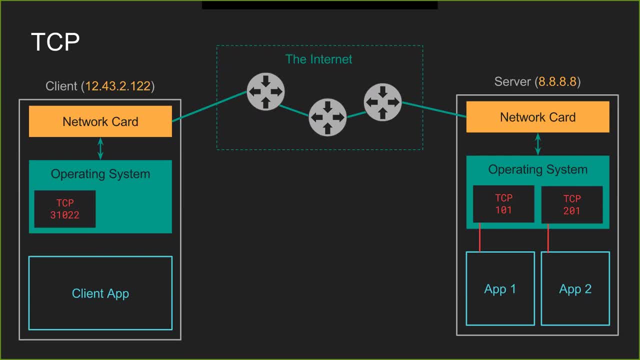 So the operating system, like it, doesn't tell the client about this, but it randomly picks a client port for it. I'm using the same numbers here. The operating system will then send a packet being like: hey, please can you open up a connection with me? 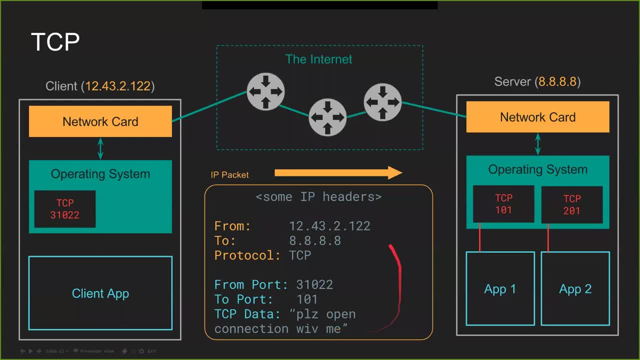 Here's my client port, Here's the port I'm trying to connect to. So it looks very similar to UDP, Except it's got this very specific message and it doesn't actually look like this over the wire. This is paraphrasing, but you know artistic license. 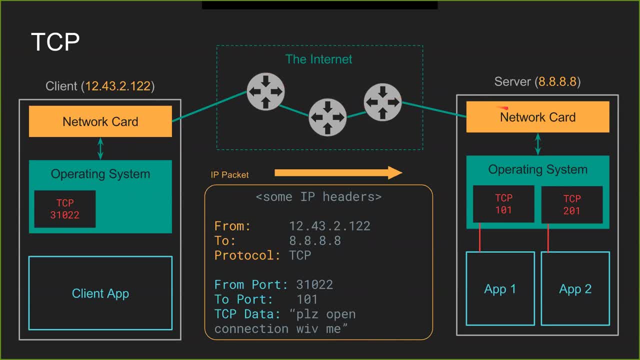 So this message goes over the network, reaches this network card, reaches the operating system and it sees this message being like this: This client wants to open up a connection with me, So then, so, so if, in this case, I'm going to support one on one, 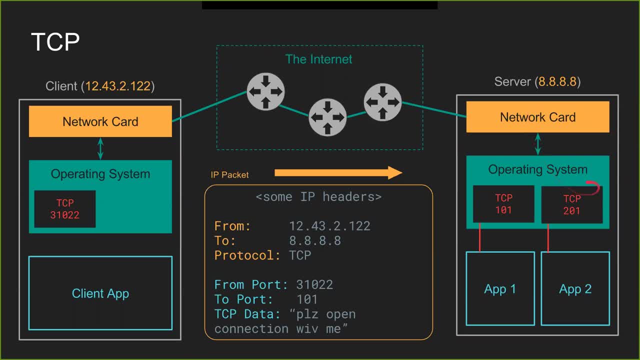 if I was trying to connect to a different port or a port that wasn't didn't have anything listening to it, this the server might send a rejection message like I refuse to open up a connection with you, which is what you get. I'll just quickly show you if you go to like. 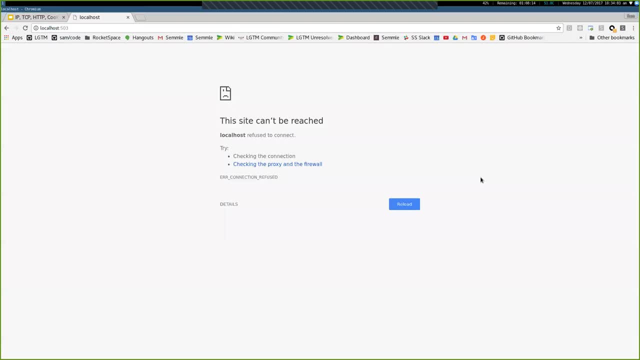 Something that doesn't have a port open. Local host refused to connect. What's happening in here is: you're trying to send a TCP connect. You're trying to open a TCP connection to port 503 on this host And it's come back with message being like nah. 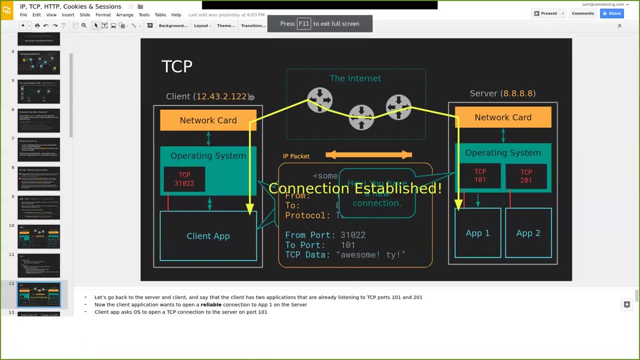 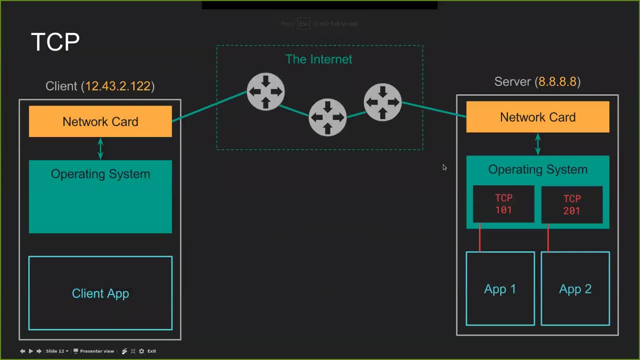 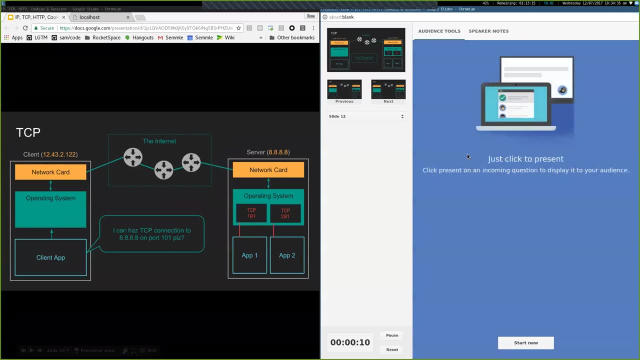 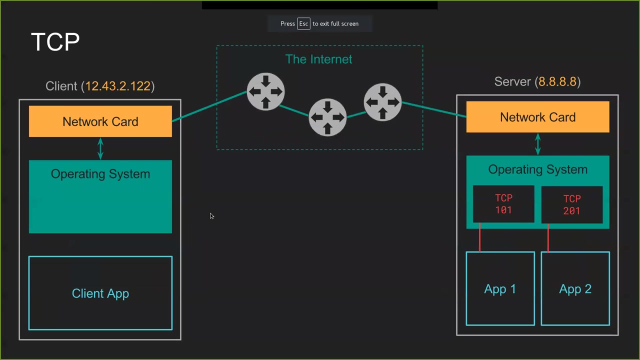 So I need to present Now. did I cancel the present? OK, I need to just Give myself my notes again. Pro tip: do not cancel the slideshow whilst you're giving the slideshow, All right? So So it sends a message being like: hey, I want to open up a connection. 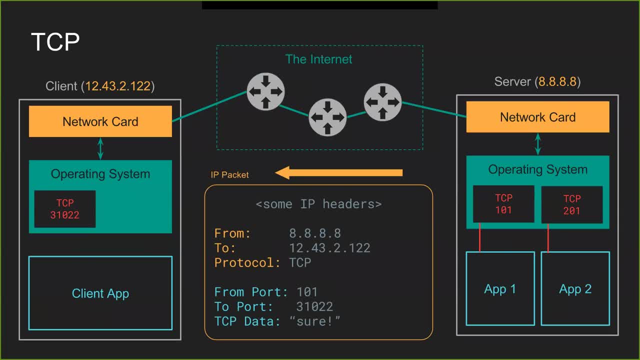 The server responds being like: yeah, I'm listening to one on one, I'll accept that connection. So it sends a message being like: yeah, sure, go ahead, Let's, let's get this started. And then the operating system is like: huh, great. 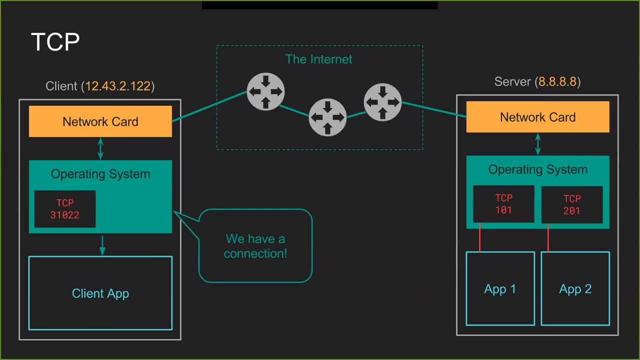 So it sends a client up being like we have a connection, Now you can start sending data, But before it actually sends the data, it sends one final packet, Say Awesome, Thank you, And that's like the end of the handshake. 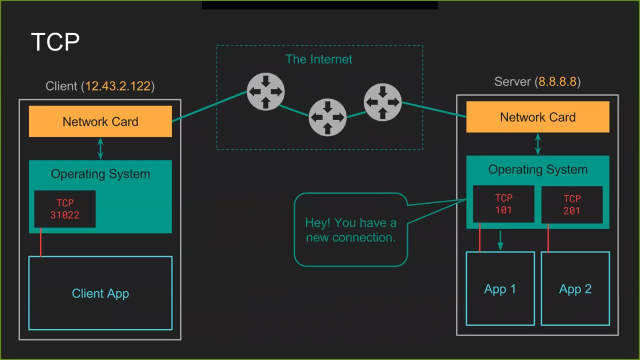 When the operating system receives that packet, it then tells the application that's listening and accepting connections on that port. Hey, we have a new connection, At which point that application can also start sending data back to the server. We can also start sending data back the other direction and we'll start receiving the data from this new connection. 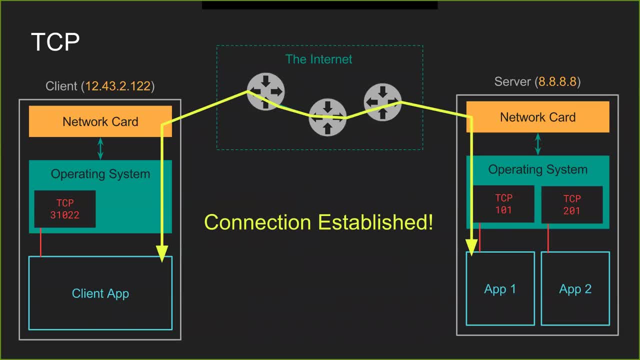 So Connection established, We can start sending data back and forth And it's reliable, because all of the unscrambling stuff is handled in this protocol by the operating system, And it's great. This is very useful. We will use this in a bit. 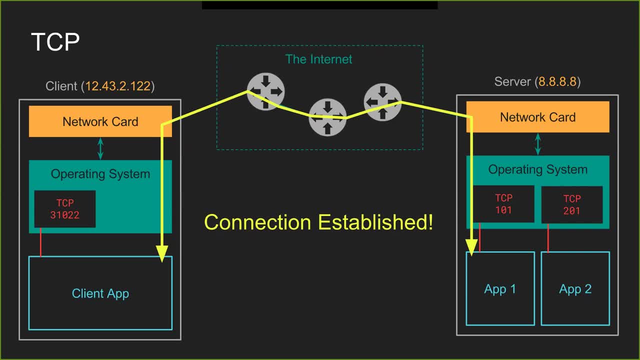 Are there any questions at the moment? Yeah, So like when you have Applications, Video And Chat? Yeah, Or does that mean they're using Right? Generally, They'll have different ports open And Multiple connections Open. 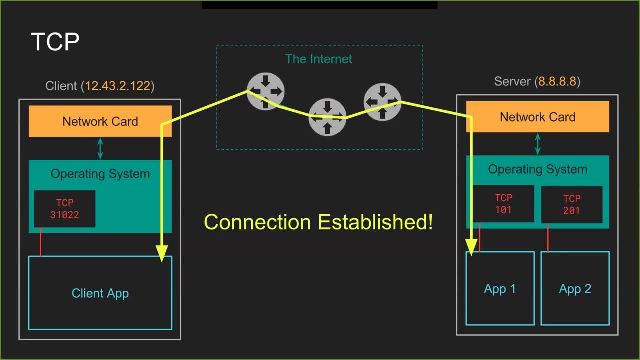 At the same time. Yeah, Cool, Right. So Slack, If you, If you use the video call or voice functionality on Slack, It's actually a little bit different, But I won't go into why. But yes, That's basically what's happening. 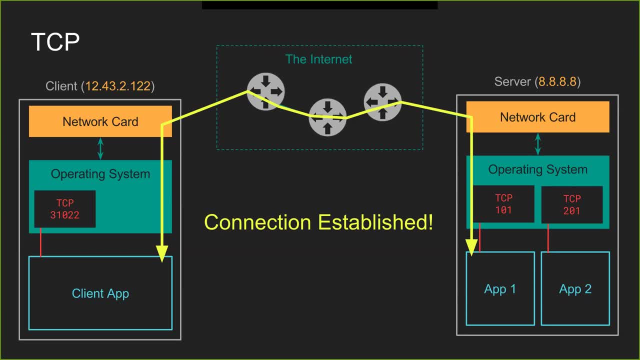 You have. You're using TCP for the chat part, So you're using UDP for the video Parts And the voice parts, Cause it matters If You incorrectly Receive text And it doesn't need to be there Like. 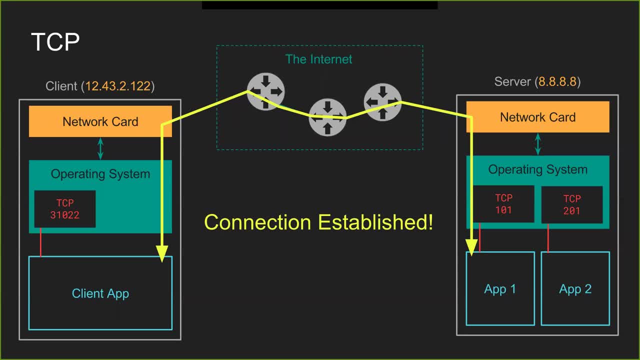 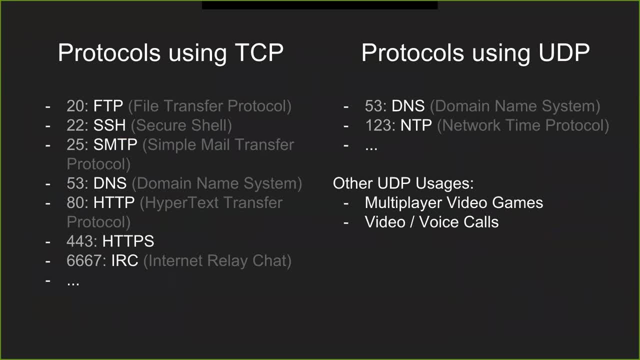 Yeah, Yeah, Yeah, Yeah. So here are some protocols that use TCP and UDP. How many people have heard of FTP? Cool, Who wants to explain what it does? Okay, Do you want to elaborate more? Right Yeah, It's a file transfer protocol. 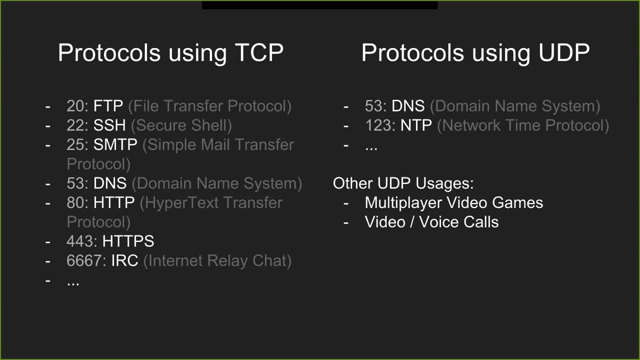 It's in the name. You upload files- Generally The most common usage hosting provider like GoDaddy- and you want to upload files to your website, you'll use FTP. don't use this anymore. it's insecure. everyone will be able to view your traffic and manipulate it. there are other things you can use. 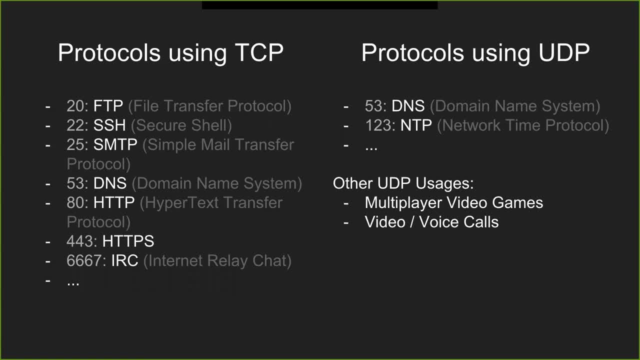 instead SSH inside of. who's heard of SSH? cool? who wants to explain what that does? yeah, right, so that's one of the things you can do with it, and ultimately it- it conceptually- connects to securely- yeah, connects to- another computer and then opens up a terminal, a shell, on that device that you can then use like you. 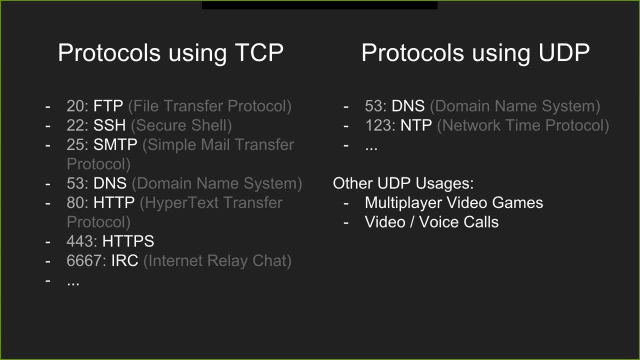 can with your terminal application locally. you can also do file transfers over secure shell. so an alternative to FTP- and it's secure- that you should be using is, I think it's ftps or SFTP- I forgot which way around is, but that's basically file transfer over SSH. yeah, if you've ever used SCP, that's an. 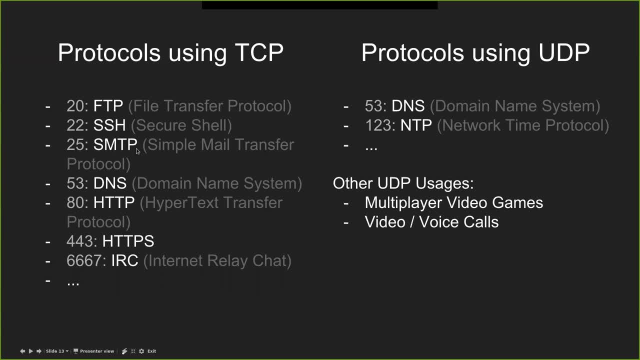 application that does this SMTP. who knows what SMTP is? yeah, email, yeah, it doesn't say in the name at all. yeah, this is. this is how email servers communicate with each other to send email DNS. we're going to be going into this in a bit, but who knows what DNS, or who's heard of DNS, firstly, and who knows what it is? 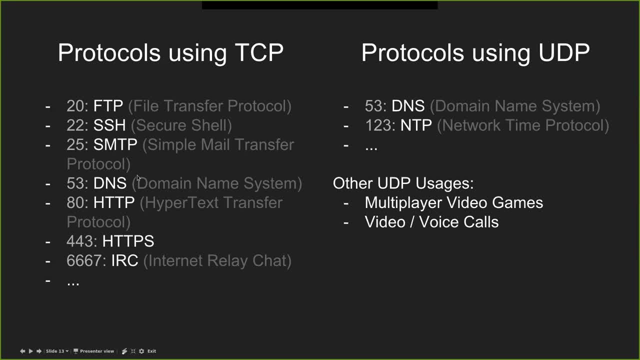 awesome, cool. hypertext transfer protocol. who's head of this one? right, this is literally like every day here. right, dealing with HTTP. who's head of HTTPS? cool, what is that? a secure version, nice. who's head of IRC? awesome, no one. this is what this was. what slack replaced? there's like 20, 30. 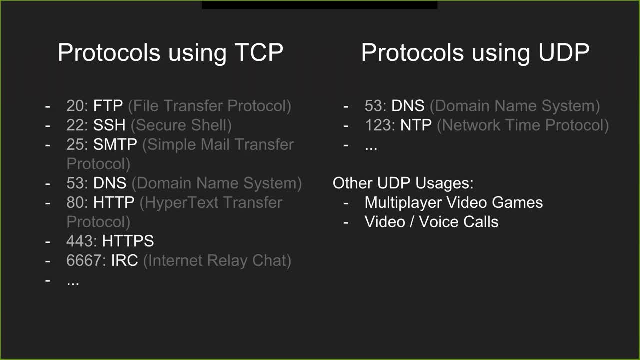 years old. in essence, that's the short way of putting it. IRC people- people that still use IRC- will disagree with me, but that's basically what slack is. yeah, nice, awesome. yes, we have some IRC users. cool, you can still use it. you can use it with slack. 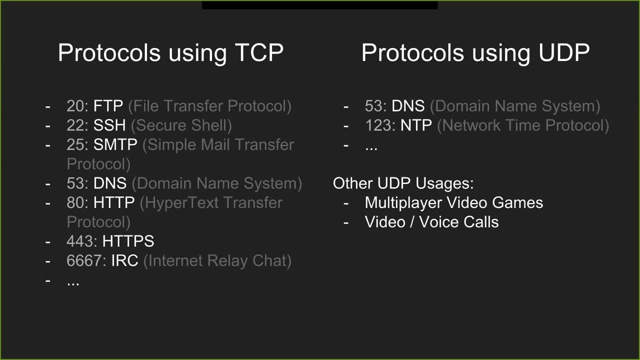 slack has an IRC gateway. if you refuse to use slacks UI, you can connect us like using IRC instead, which many people do, especially at my work. about half the people at my office refuse to use slack, so they still use IRC but connect to slack. cool, UDP and DNS uses UDP as well. it uses UDP and TCP. 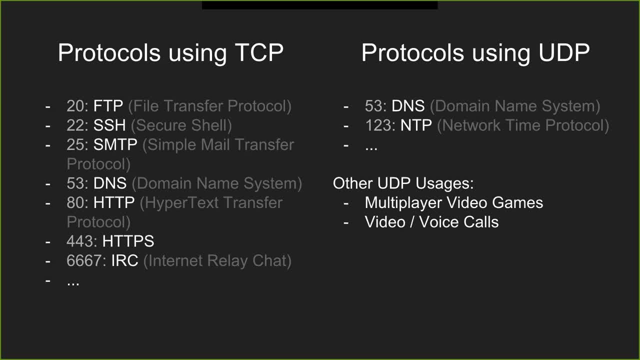 does anyone know what NTP? I had anyone heard of NTP. yeah, who knows what NTP is, then wants to guess by the name what it is. what does it mean? what does it mean? it's basically working out what the time is where you are. so every device in this 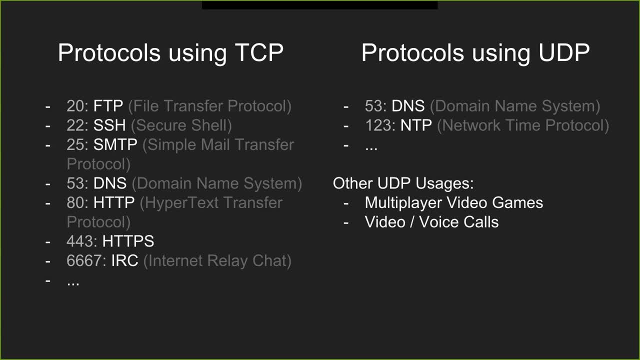 right all these max at the moment, but the thing is this is pretty limited on the. They're gonna be doing this- all your friends are probably gonna be doing this- by communicating with some upstream server, Like hey, can you tell me what the time is? and then it says a mystery, like the time was about this, which is why. 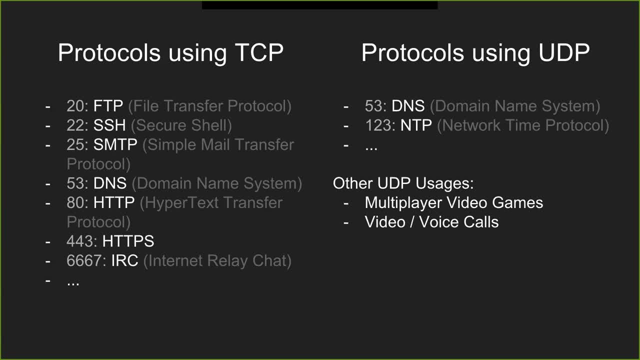 Pretty much why we have such a good timekeeping now, Like you never need to really like change the clocks like you used to, unless you still have analog clocks that aren't connected to the Internet, Which you should do because they're awesome, Right? So if it's internet-connected, 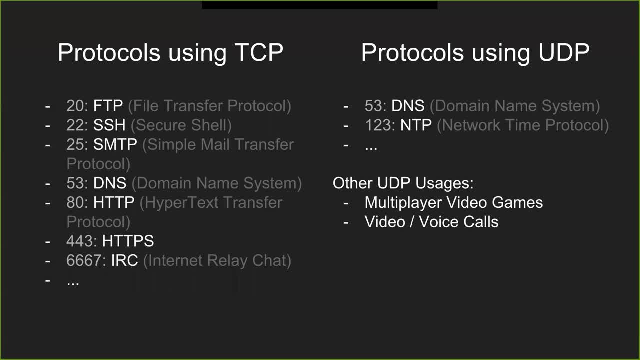 It's because it's using NTP. if it's something that isn't internet-connected, It's generally because it's got a small backup battery But doesn't actually just keeps the time going. So, for example, if you have a, if you have a laptop, 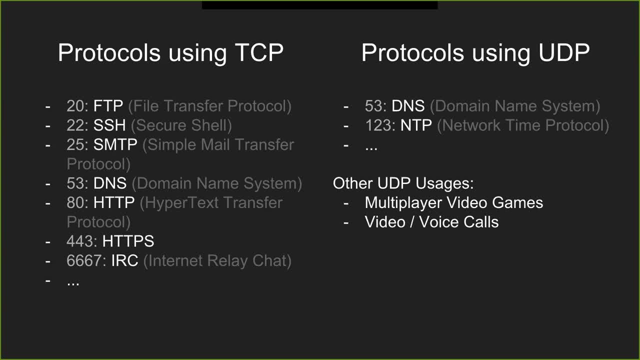 And you take the battery out and you take out the network card, don't connect to the internet at all and a couple years later plug in the power again. Time will be Roughly about right. And that's because it has a no start-ups. have a battery inside. That's surely for making sure the clock keeps going. 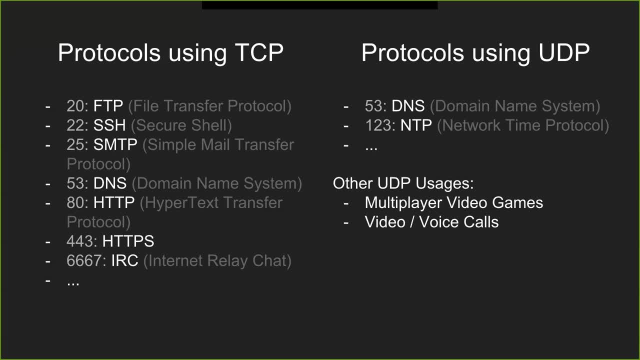 If you've ever opened up a laptop or even actually desk desktops, have this as well. on the motherboard You have like a little, a little battery That's purely for the clock. So if you ever- if you ever like- built your own computer or open up a computer, you might have seen one of these. 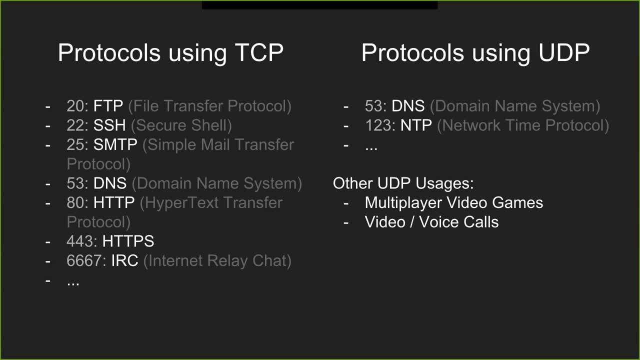 Has anyone seen this battery? No, Yes, over there. Yeah, the little circular one that you normally get like it's like a watch battery, Yeah, Cool. and then UDP is used for things like multiplayer, like games and lots of proprietary stuff like Skype, etc. 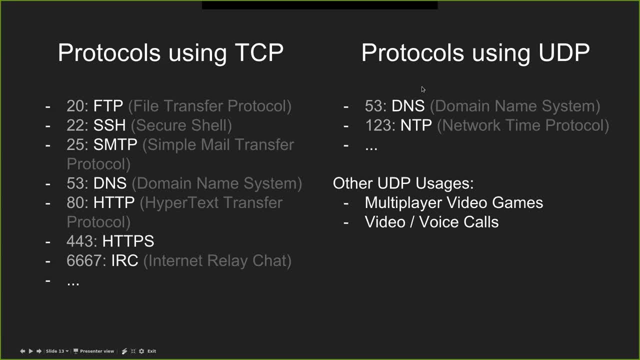 Where are we? time-wise? 1042. All right, I actually feel like I have done enough content preparation. Oh, almost now we're reaching the end, cool. So what do we have at the moment? So we have a way of identifying devices on the internet. 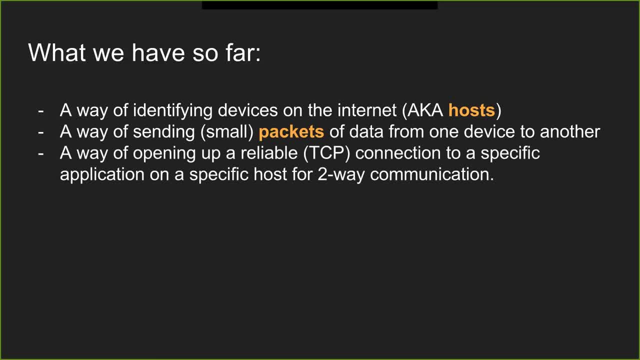 We have a way of sending Small packs of data to those devices. We have a way of opening up a reliable connection to a specific application on a device, say the devices hosting the website. Is this enough technology to ask for a web clip, for a web client to ask for a specific web page? 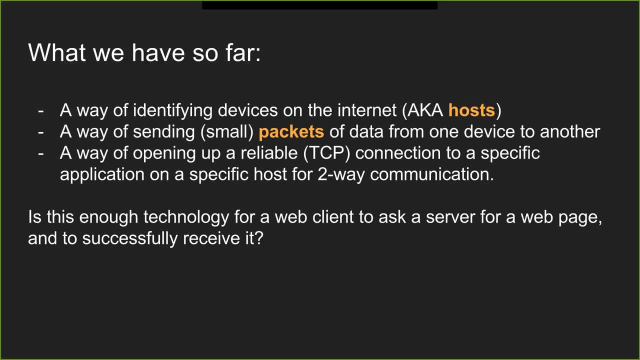 Who thinks yes, raise your hand. Who thinks no, raise your hand. Who doesn't know, raise your hands. if you didn't raise your hand, raise your hand. All right, cool For those remote. Basically everyone didn't say yes or no. There are a few people that did and the answer is no. we haven't got enough stuff yet to later. web page. 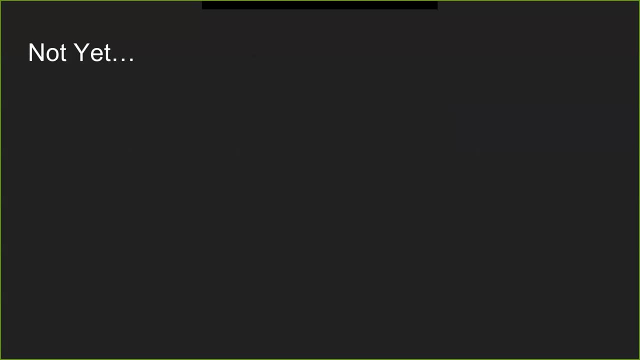 We need to introduce a new protocol. Actually, there are a couple things we need to do. firstly, We need to know how we get from domain names to the IP address. How. how do we know the githubcom, or how do you know the IP address of the server That's hosting? 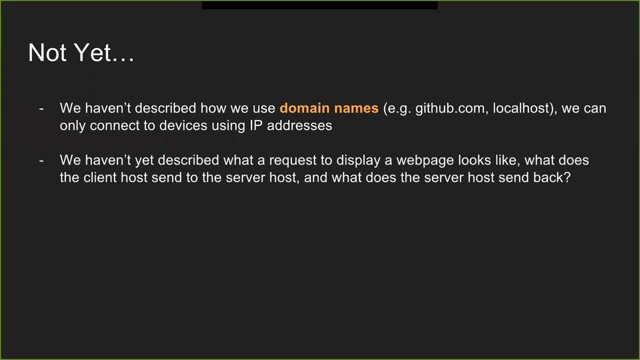 yeah, and then. Then we still need to define this protocol, which some of you might know the name of, But I'm not going to actually say it yet. cool, Say again, That's the. that's the first one. That's what we're going to address right now. 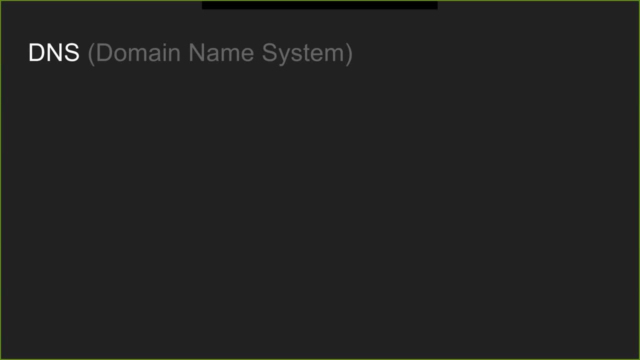 so domain name system. You can give me a quick description of what this, or who thinks they can give a description of what this is, before I say it the domain name, and then it's: Yep, that's basically it, and it's a really complicated and elaborate system, but I'm gonna try and give you a basic overview. 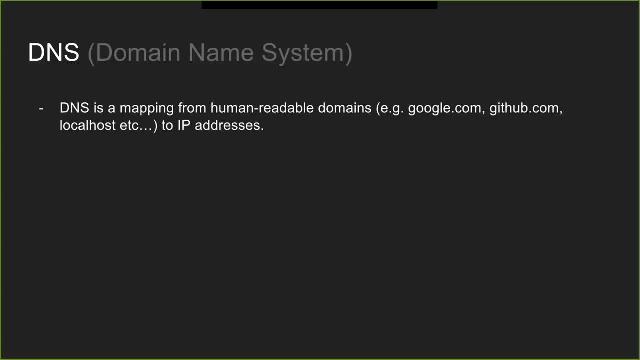 All right. so it converts domains to this. It also includes details of how to send emails to people, to things in the particular domain, and these are called MX records. So if, as an application, you want to send an email to a user, It's not like the normal way to do it. 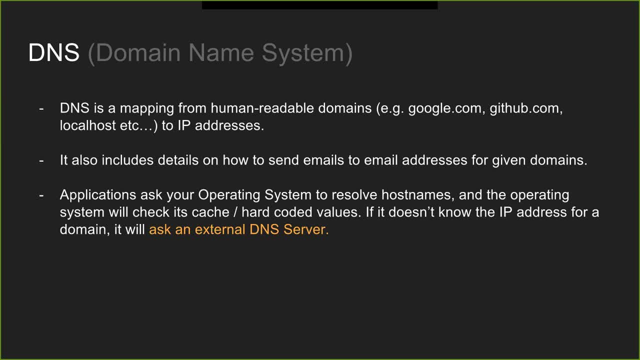 You want to connect or you want to find out what a specific IP address for a host is. You know. you ask your operating system, like with everything else, like you want to open up a connection, You want to send data, you want to know what the host is, or the IP address. 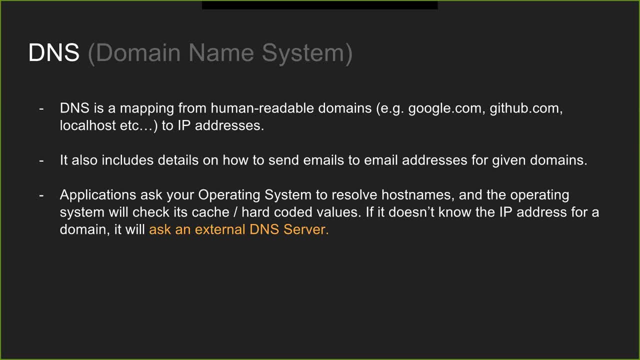 You ask the operating system, and your operating system will check firstly any hard-coded values that it has, If it or, and then it will check its cache, because if it's, if you've made a request recently, It might still know, or think it thinks it might still think it knows, what the IP address is. 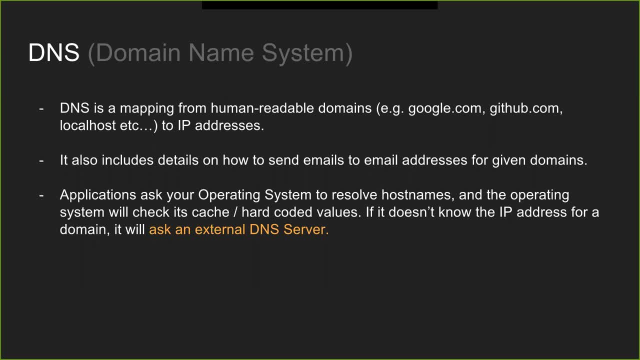 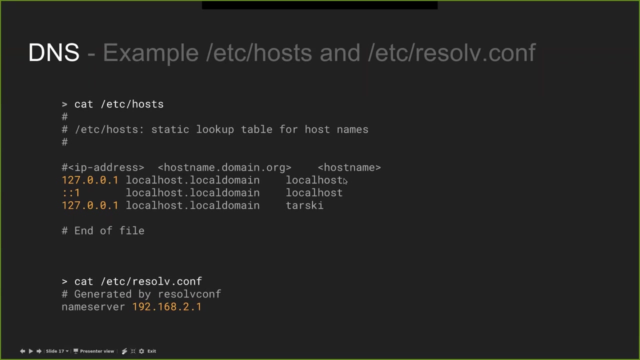 If it doesn't know, it will then ask an external server In Mac and Linux. you can open up this file And what that is is a list of all the hard-coded DNS entries. So Here's what mine looks like. you might recognize this bit of text here. who's seen this before? 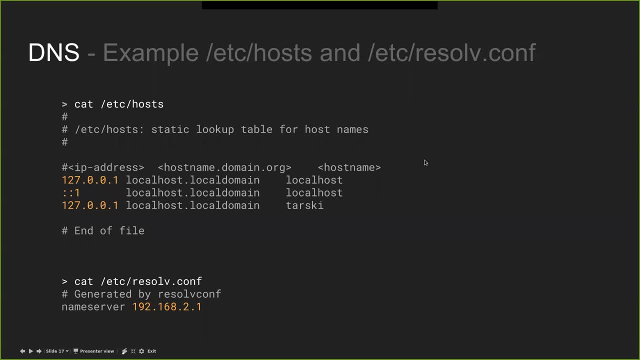 If you're not raising your hand, you should probably be raising your hand, So one of the. so I Mentioned briefly earlier about the fact that you have multiple network cards or you. you can't have multiple network cards. some of those. so, conceptually Some of those network cards are physical cards, like the wireless card, the Ethernet card. Some of them are virtual and they're in software. 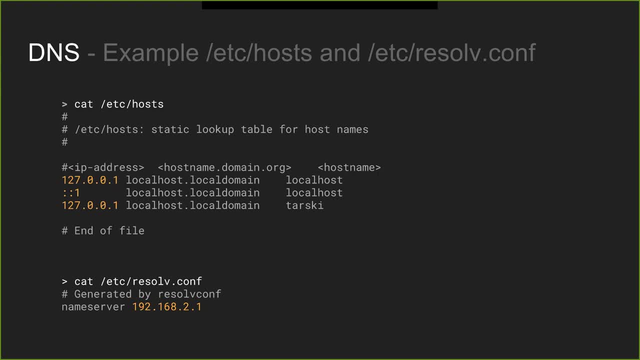 one of them is what's called the loopback interface, which is basically a way for your operating system to pretend that it's on a network even when it's not on a network, or even if it isn't a model network, and it always assigns itself a particular ip address, and that ip address is 127.0.0.1. 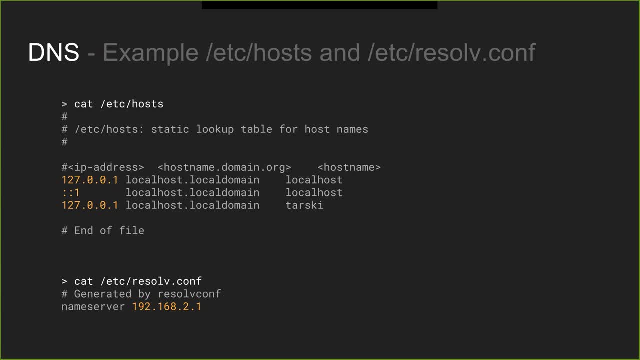 which you may have seen before, and if you really really want to, you can change this behavior. um, but don't, there's no point doing that? um, this is a standard. this is what, how it works on pretty much every machine: windows, linux, bsd, mac, android, ios, palm pilot. 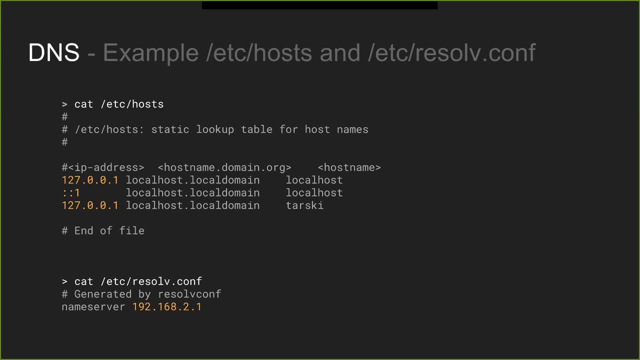 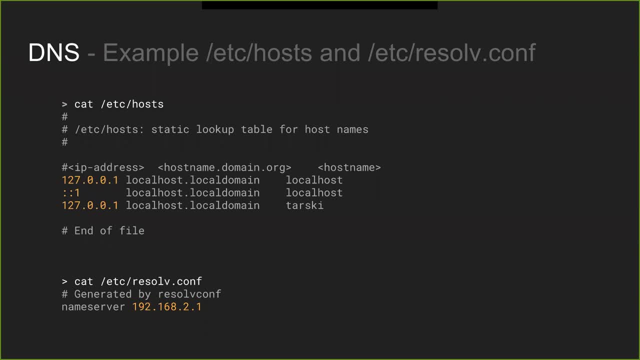 is the better, um, and what this allows? what this actually allows is for applications, all on the same device, to connect to each other using tcp, using udp and any other protocol that's built on top of ip, which is what happens when you visit localhost in your browser. 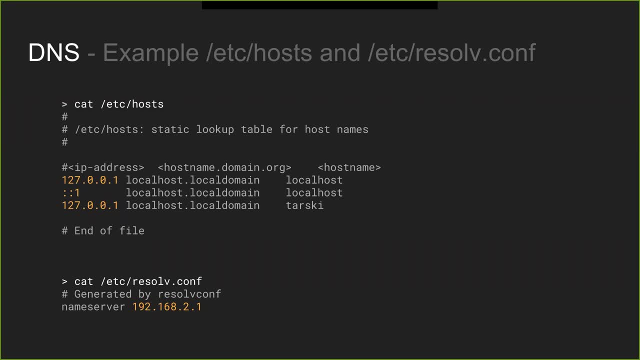 so, um, like, as a web browser, you want to like, connect or view a certain, like view an application that you're running locally. it sends a request to the operating system like, hey, i want to connect to this ip address, and your operating system says, oh, that's. 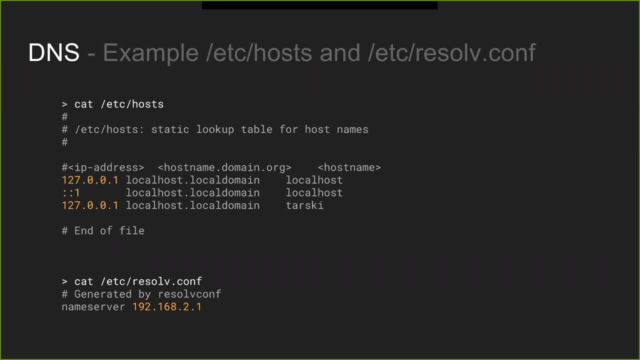 me, have i got any applications that are listening to this port? and if it has, then it then sends it over to the right application. cool, uh, yeah, so i just did that in the timeline and i see broadcast. um, i will need to look at it to be it, but i can look at that afterwards and 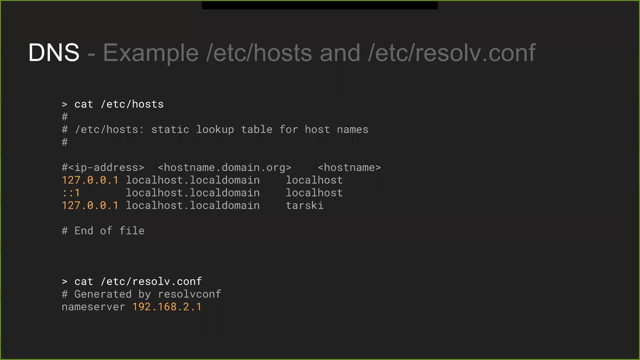 figure that out. um, yeah, things are a little different. um, this is linux, so things are a little different. um, and then there's also this other file here which oops, which exists on mac but it isn't used. but i'm going to talk about it anyway. um, and on linux, this file basically tells you: 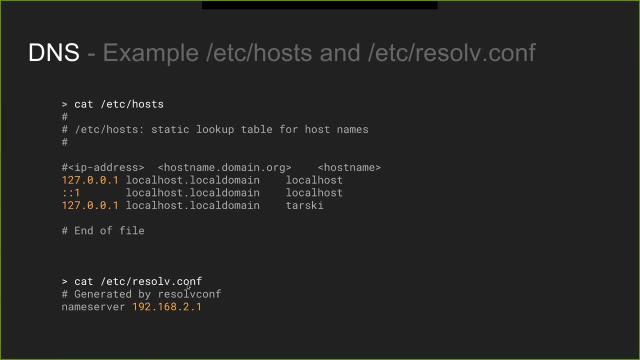 the ip addresses of the external dns servers that you're going to ask for information if you don't know what the host is. say, for example: so if i'm trying to connect to githubcom, um, or i have an application on my computer that's trying to connect to githubcom, for example chrome, it might be git, it might be ssh. 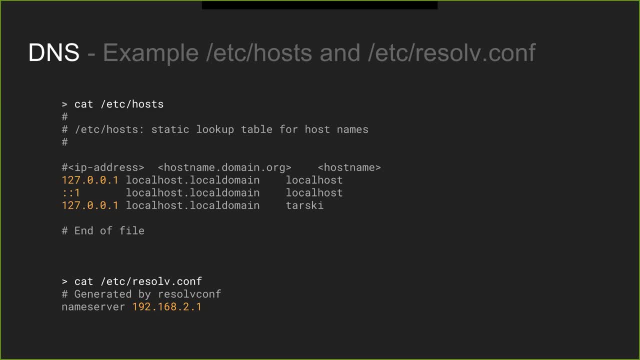 might be something else. so ask the operating system. hey, do you know what the ip address of githubcom is? my operating system first looks at this file. it says, huh, i don't have, i don't have anything hard-coded. then it looks at this files like: do i know anyone i can ask to find? 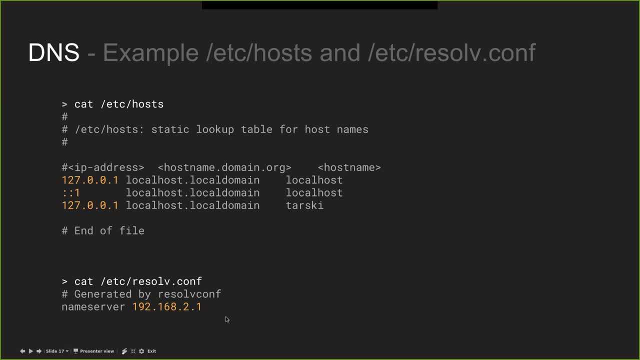 that information and this file says yes, this one. so it then sends a dnf file to the operating system and it sends a dns request, a dns packet, um over udp to this ip address saying: hey, can you give me the, the, uh, the, the ip address for this um, host this. this server will then check its own cache. 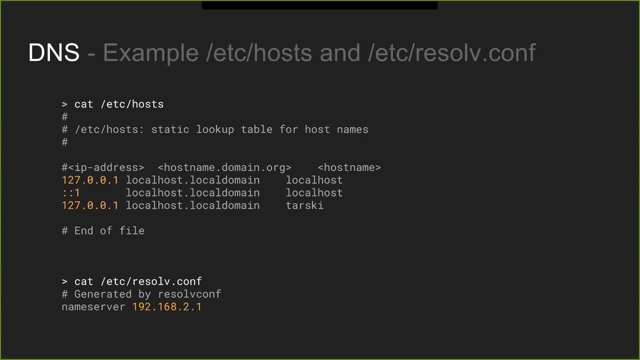 and its own hard-coded value to know if it knows anything, and if it does, it sends it back. if not, then it sends it upstream, and that keeps on going until you reach um, a particular server called a recursive dns server that will actually do that, and then it will send it back to the server and 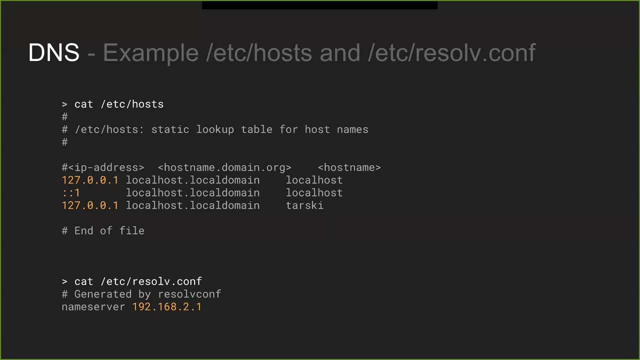 actually do the calculation for you, um, and i feel like i need a whiteboard to fully describe what that is, but i can go into details if people are interested later on about how dns works. um beyond, you want a host name and you get an ip address, but that's ultimately all you need to know. i just 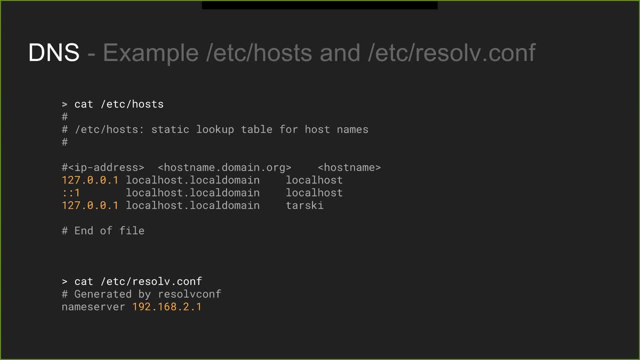 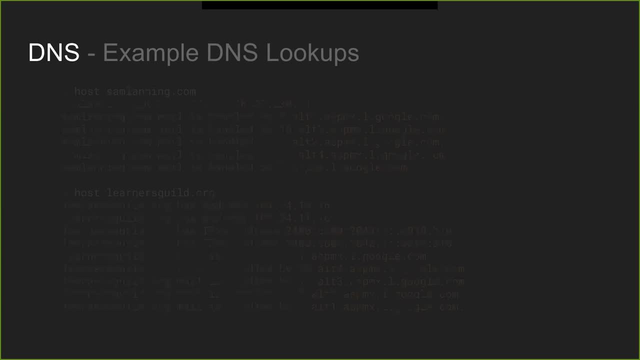 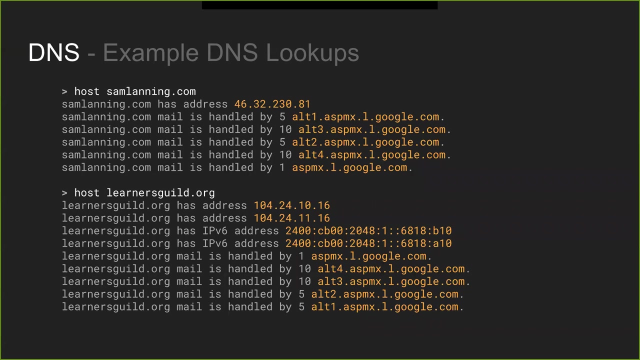 went into way more detail than was required. um, cool, so we have 10 more, 10 more minutes left. all right, here's so you can do a dns look up from the command line. um, i don't know what the command is on mac, but on this is a common one. so here are two examples. what's so? i say: give me the dns record for. 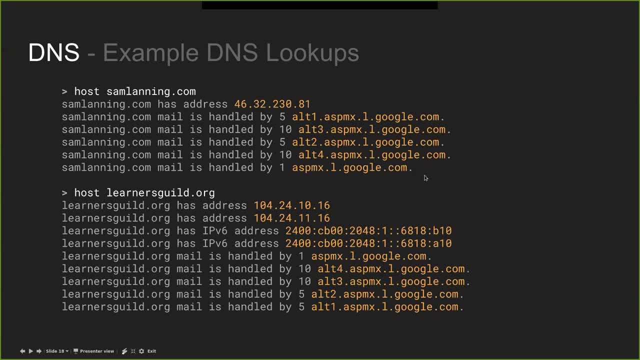 samlanycom. it says: this is the ip address and this is: this is how you send mail and i'm using google apps. so, like learners guild, here, you can see that google handles all of my email, because creating servers or running servers that handle mail is like one of the most annoying and 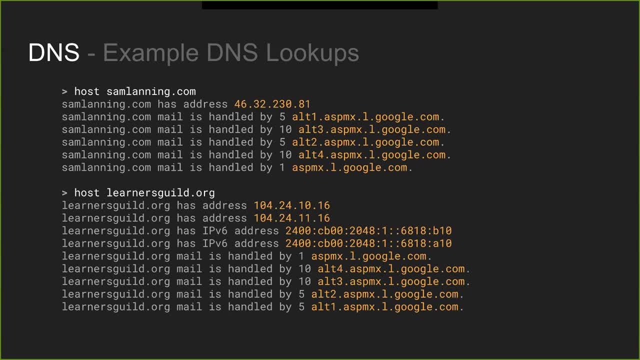 painful things to have to do as a system administrator, so let google do it. basically, um. and then, yeah, learners guild. learners guild is interesting because it has two ip addresses that it gives you. um. what this means, uh, is that, um, both of them should work. and the, and it's free. and the. 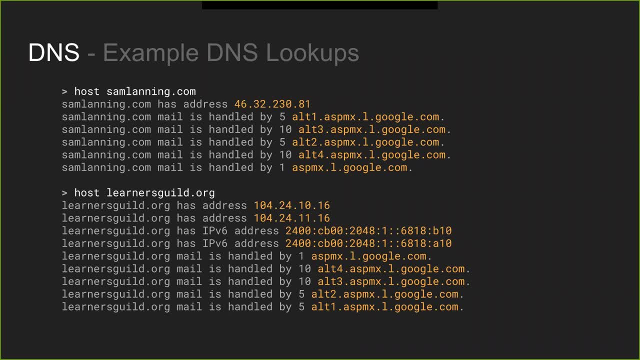 the client is free to pick whichever one it wants out of the two. um. usually clients pick the first one. um, there are a number of reasons for this. um. has anyone heard of load balancing? you can raise your hand if you have. yeah, cool. does anyone know what load balancing is? 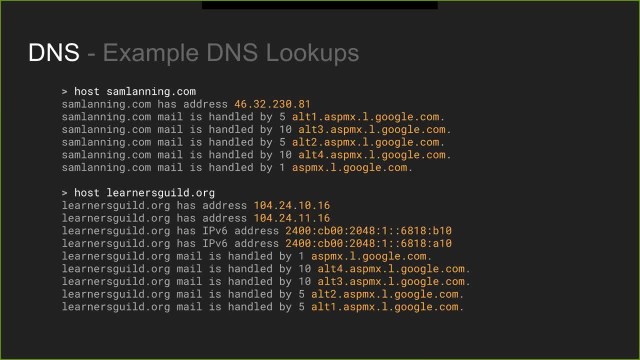 yes, right, it's spreading, spreading for this um, so for store or representative with this. uh, it's for working on a task or something like that and for your rowing table that you can track the task and track. it's a fairly complex thing for a load balancing, um, and it's it's also a very interesting way to. 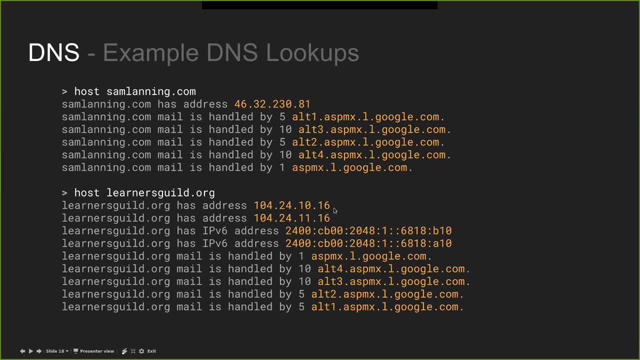 sort of represent the way you ask a request. yeah, and this is a really interesting feedback as well, which is that you can rely on the data that you have, you can hand it over to that taskmaeter and it can be used in the same way that you would would use a request on a task. 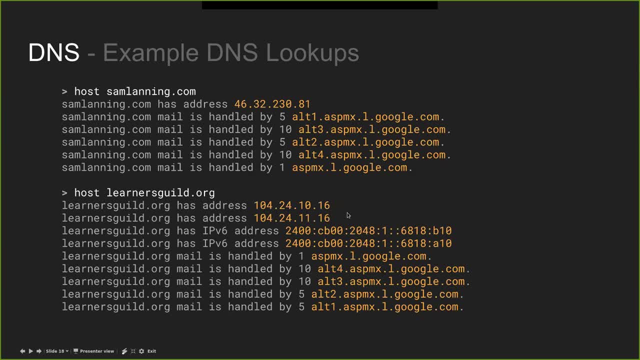 um and um. you've got a lot of common things going on with traffic over multiple machines that can receive and handle appropriately handle that information. so giving multiple ip addresses back um is one technique that you ask for a request so that it's more likely that people will be going to. 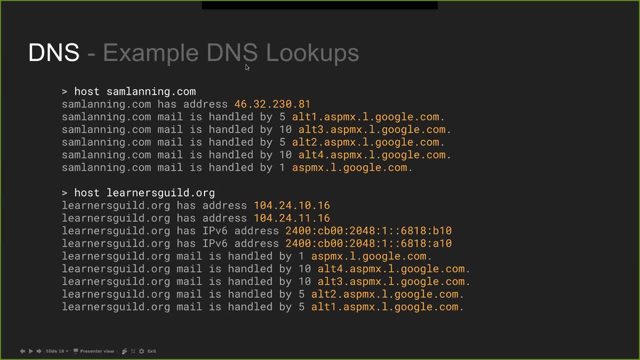 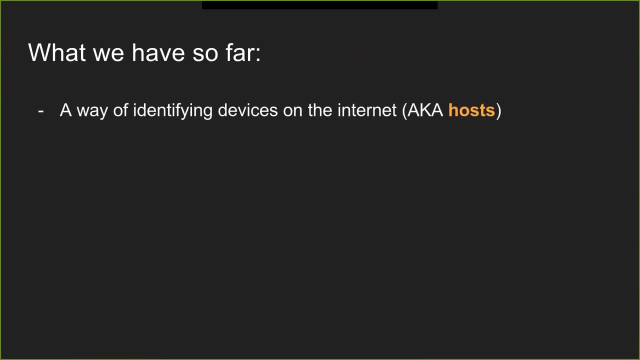 different IP addresses rather than everyone still going to the same one. cool, all right. so what do we have so far? we have a way of identifying hosts on the internet. we have a way of sending small packets of data. we have a way of opening up a reliable connection to one of those devices. we have a way of 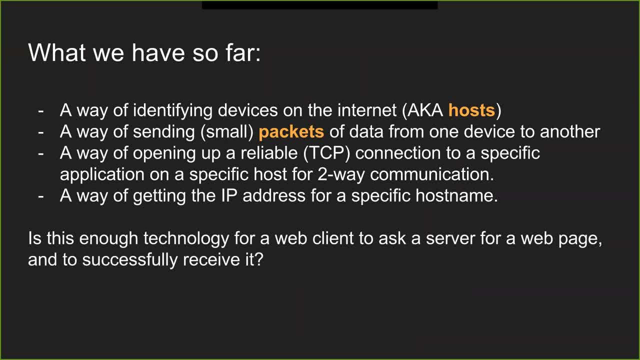 getting the IP address for a specific host name. is this enough to load a web page? raise your hand if you think it is. raise your hand if you think it's not. raise your hand if you don't know. raise your hand if you didn't raise your. 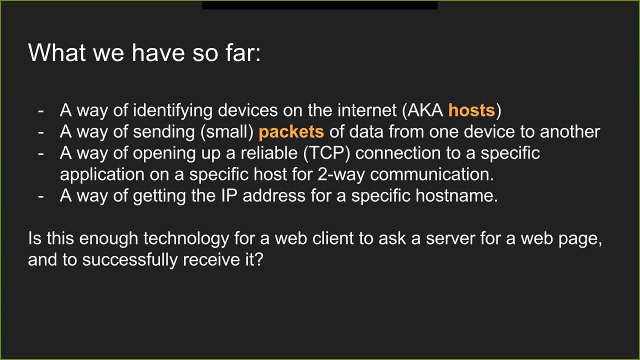 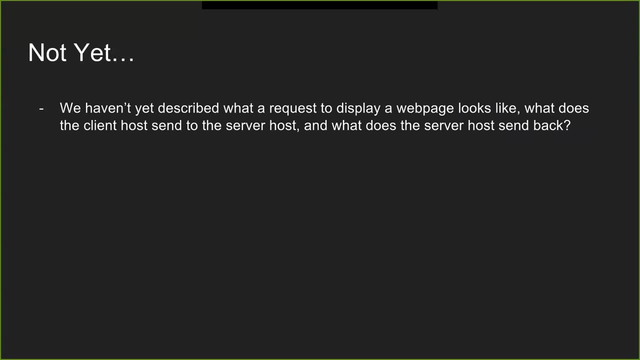 hand people. this is not. this is not how you raise hands. you need to like, actually lift it up and defy gravity. all right, no, we don't have enough stuff yet. we haven't yet decided. described how what a request to display a web page is like. what do you send a? 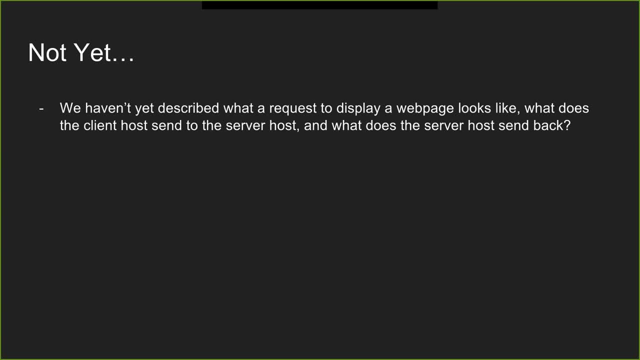 server when you're like I want to view this web page, and what does this ever send back? anyone know what this is called, but we're about to go into I'll give you a clue. it starts with an H, yes, yes, HTTP hypertext transfer protocol. who can tell me what technology they think this is built on top of bingo? 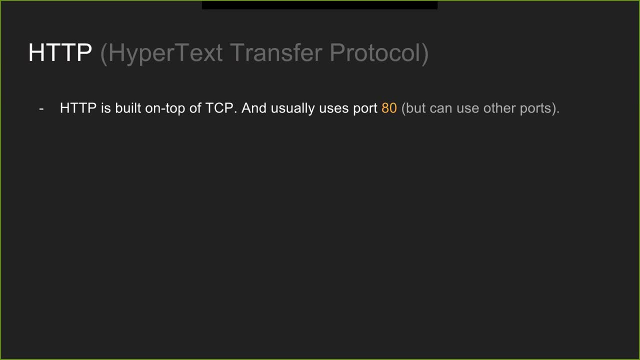 HTTP is built on top of TCP and the standard port I use is port 80. so when you have a web address in the browser and you don't have that colon and then some number, port 80 is being used. when you do have it, it's using a different port. so I'm gonna take a risk: damn it, no, I'm gonna. 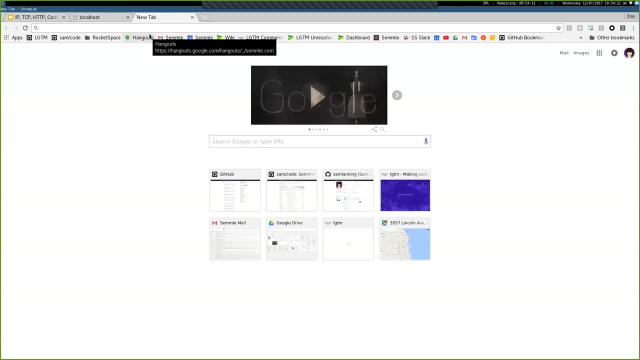 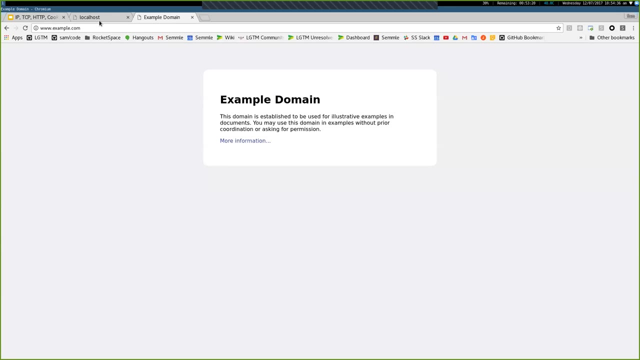 have to restart. okay if say, if I try to go to what's a good one, okay, no, that one won't work either. okay, let's do asdcom, examplecom, that exists, samplecom, all right. so examplecom is a website that actually exists. it's actually a reserved website purely for being used as an 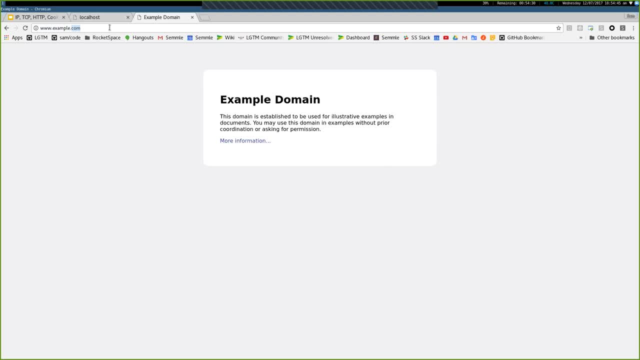 example. it's kind of like the politics around examplecom is kind of interesting, but you legally you're allowed to use this in documentation everywhere. it's like copyright free. you can paste it in link to it and it's fine. if I try to specify, I actually want to go to port 80. 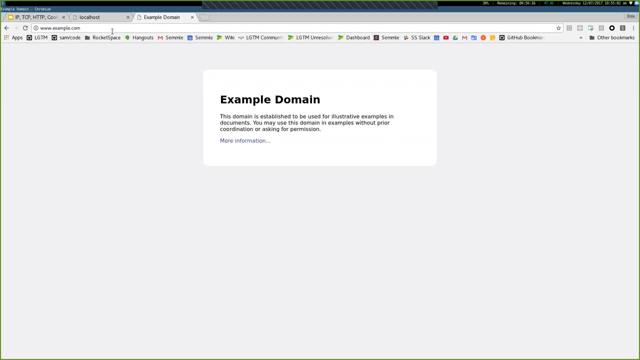 like, specifically, chrome will hide it away because it's the default port. like, well, obviously you want to go to port 80, that's the default. if I then say I want to go to like a different port, at that point chrome and same other browsers won't won't hide it because it's a non-standard. 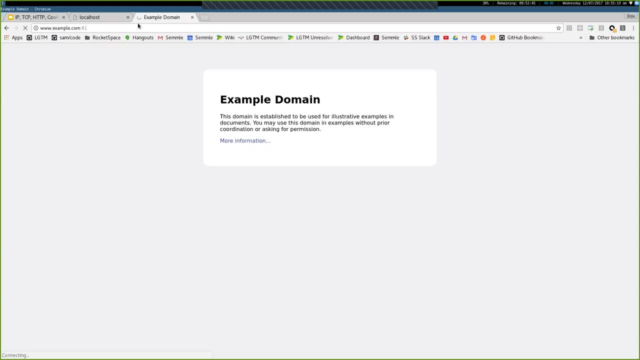 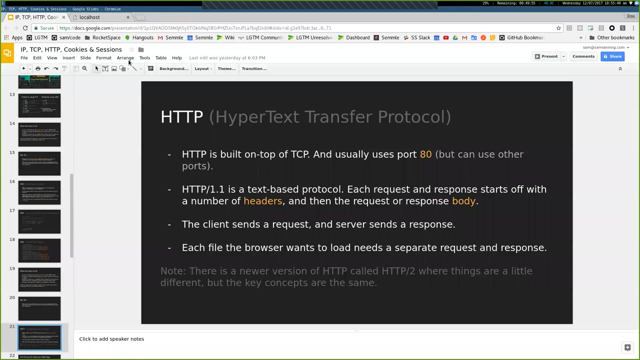 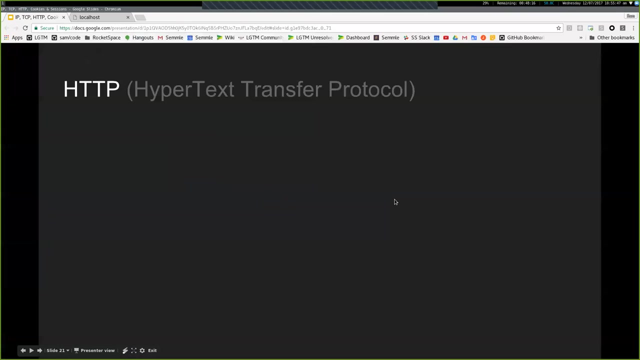 port. it's not the default port and and with https the default port is 443. so if you try to go to say google, googlecom, colon 443, it will again hide it. cool right, let's see if we can restart this presentation again. present presenter view. move that to my other window- full screen. 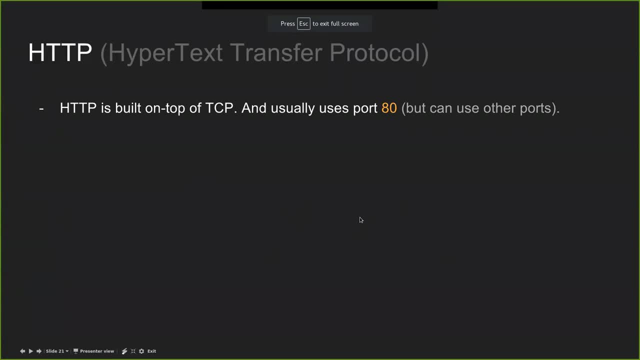 all right. so HTTP is built on top of TCP. HTTP version 1.1, which is the one you'll most commonly see documentation about online. it's supported by all the major browsers. it's supportive by all the major server software. it's the only one you really need to care. 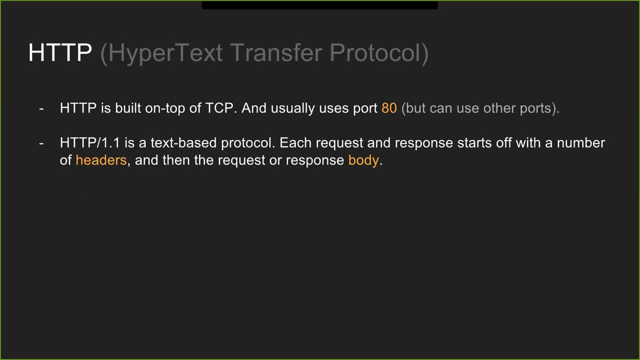 about, at least to begin with, um, and it until about two years ago. it was still the latest version. it's been the latest version for like 20 years, thinking about absolutely never be the latest version of TCP. this is not something that you're still going to have to do. for those of you who have, You have to. 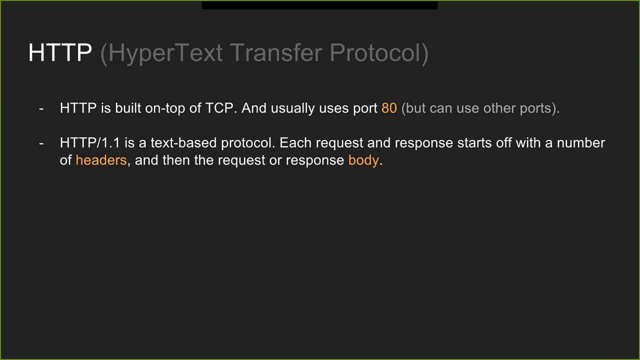 version. It's been the latest version for like 20 years. HTTP 1.1 is a text-based protocol. So how many people saw Trevor's talk on Monday or lecture on Monday? Yeah, a couple of people. Okay, So he went over what raw HTTP looked like, which is basically text. It's human. 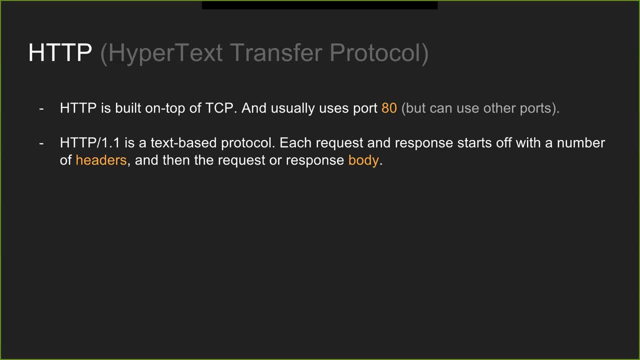 readable, You can understand it. I would recommend having a look like after this lecture, having a look at that lecture on YouTube If you weren't there to see it. it'll go like this: It'll actually go into the detail of the structure of what HTTP looks like, Way more than I'm. 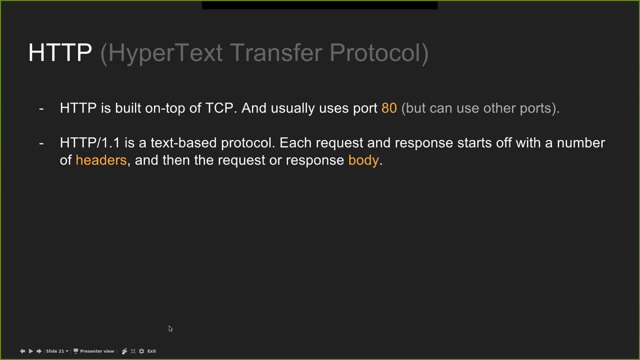 going to talk about today And, given I only have three minutes left, definitely don't have time for. So. it uses it basically like sends text over the wire text back, And each request and response has a collection of headers which is basically like metadata. 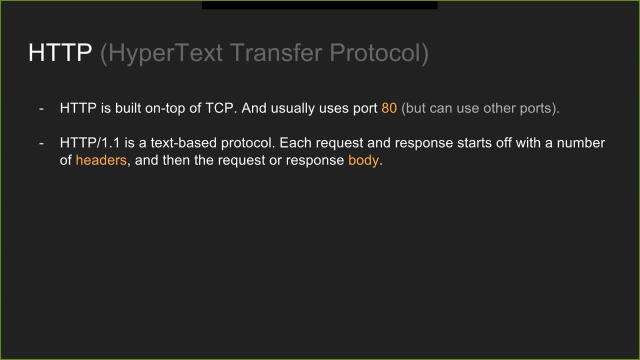 It's like an email address. it's a legal address. It's like a code for the web page. It's like a password. It's like a password. It's like a password to like a browser, Like things like cookies, things like the path, Things like. by the way, I'm using this. 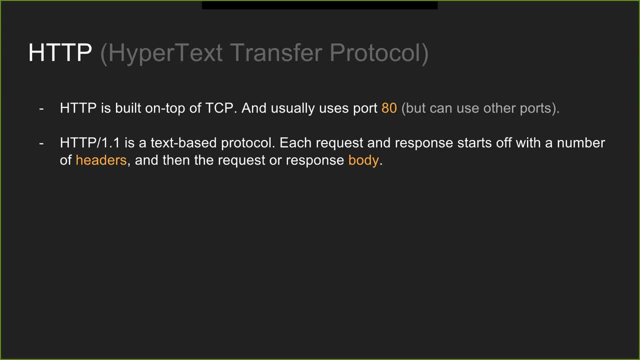 browser. Things like these are the types of files I accept. This is the language that I use so that browsers can like send different web pages for different languages. For a while, I actually only set Spanish as one of the languages in Chrome, So my language priorities. 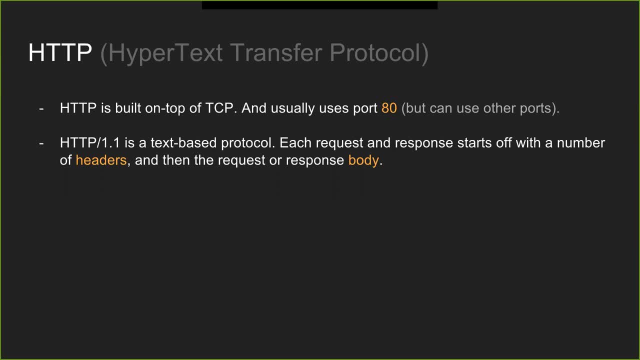 were British English, Spanish, American English, And for a while I sort of just I didn't really know what to do with these things, And for a while I had no idea why, when I was looking at certain websites, it was showing it to me in Spanish first. 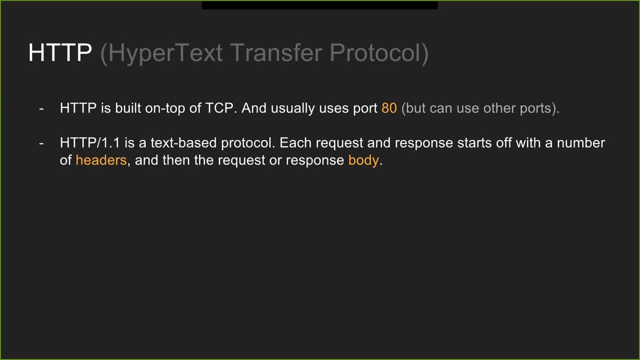 because English was my default language, right Wrong English. So yeah, websites that understood this header, this information, were giving me pages in a language which I didn't actually understand but was attempting to, which I think is why I actually changed the setting and forgot about it. 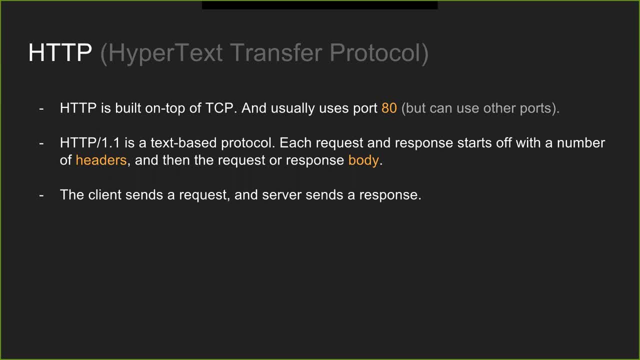 Cool. so the basic idea is: client sends a request and then the server sends a response, Each file that the browser wants to load. so you load a homepage and then you can see from that homepage that you also need to load some CSS files and some JavaScript files. 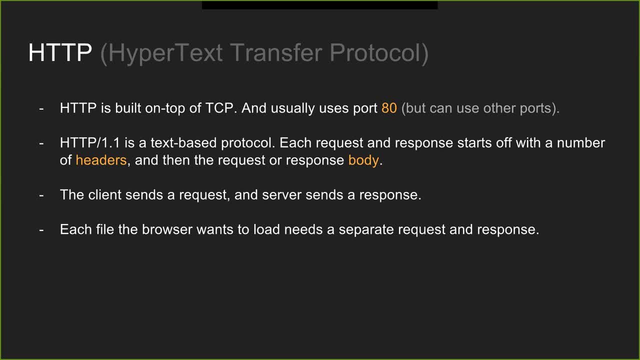 and some fonts and some images. Each of those different files is a different HTTP request. the browser sends back to the server and the server responds with that data. Any questions about that? No cool, Like side note The reason why I was talking about HTTP 1.1 in particular. 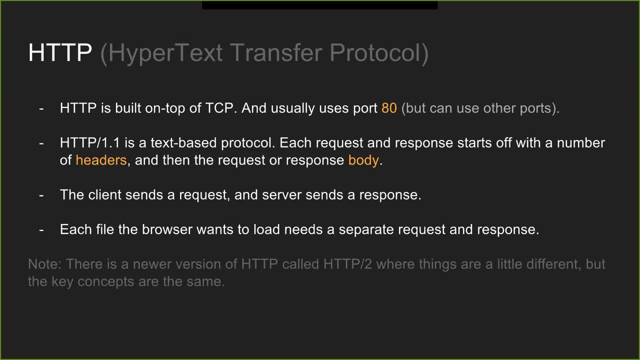 is because there is now a new version called HTTP 2.0, which was previously called SPDY, spelled S-P-D-Y, because who needs to use vowels in the tech world? Started off by Google and then worked together with various other internet companies. 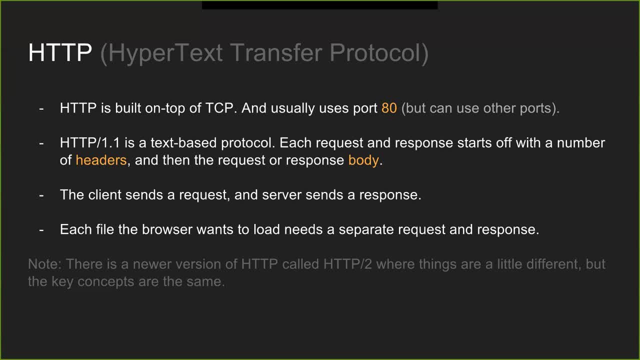 to sort of finalize the protocol and make it the official next version of HTTP. Things are a little bit different with HTTP 2.0, but it's a little bit different with HTTP 2.0. The high-level concept is still the same. 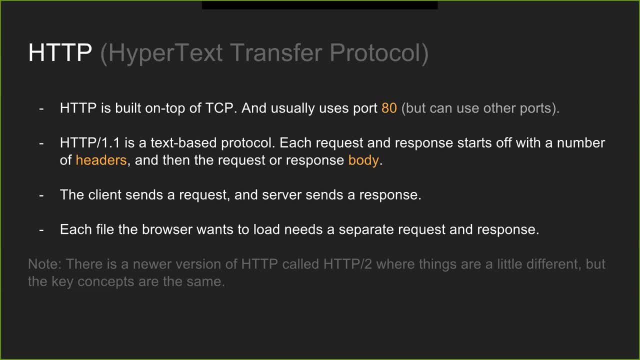 but it's no longer a text-based protocol, So you can't do the same thing. Another difference is HTTP 2.0 requires you to always be connected over a secure channel. So there's no, you can't use HTTP 2.0. 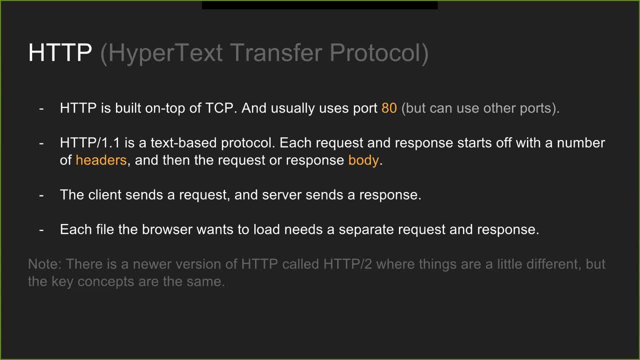 if you haven't got security set up on your server and you can't use HTTPS. If you can't use HTTPS, you can't use HTTP 2.0. HTTP 2.. There's like lots and lots of resources online about all this. it's all. 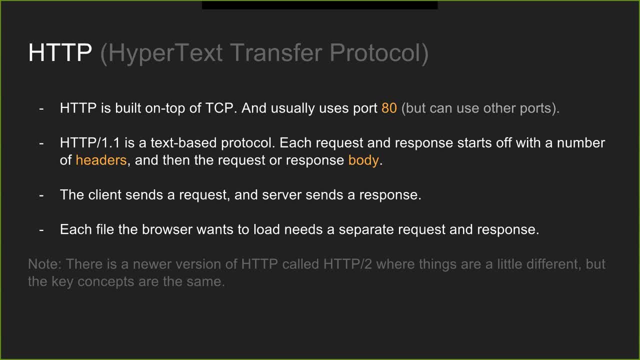 very new, so it's like pretty cutting-edge and there's some really cool features that it has. it's not necessary at all for you to know it for the for the next part of your learning, but it's interesting and it's some pretty useful stuff. we use it at my company and take advantage of it. okay, so going right back, 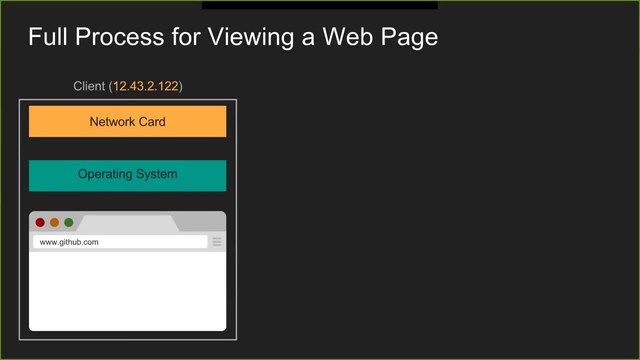 to the start. we're running over a little bit now, but I'm just gonna go back over to the high-level process. so what happens when you open up a web browser and view a web page? firstly, the web browser says: what is the IP address for this thing, your operating system? then, if it's in its cache, it sends the. 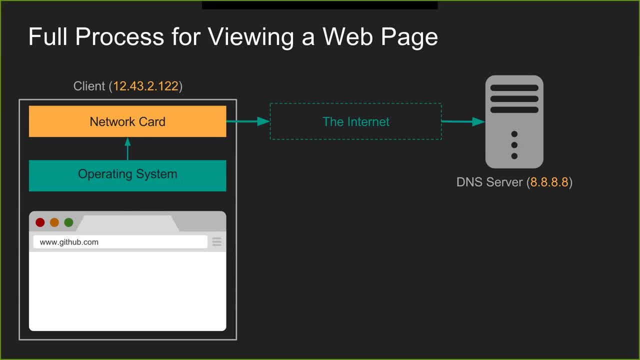 information back. otherwise it connects to a DNS server. it says: hey, can you tell me what the IP address of this thing is? the DNS server then responds: it has this IP address and the operator system sends that back to the browser. and the browser is like: great, now I know what the IP address is. now I can send a. 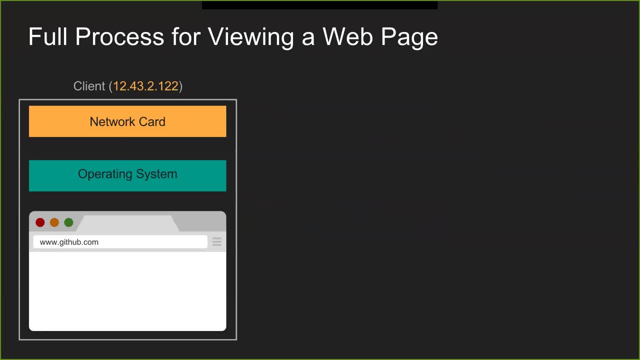 now I can connect to HTTP and actually send a request. so that's what happens next. so it's like: please can you open up a TCP connection on port 80, because that's the default port for HTTP to this IP address, which is the IP address it. 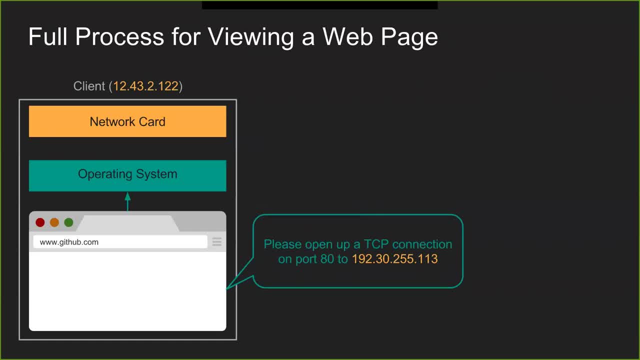 just received. that was as far as I got with the animation, so I'm gonna hand wave the rest of it. the operating system then, as we showed with the TCP handshake: it creates a client port. it sends a request like: hey, can I connect to you on port 80? the 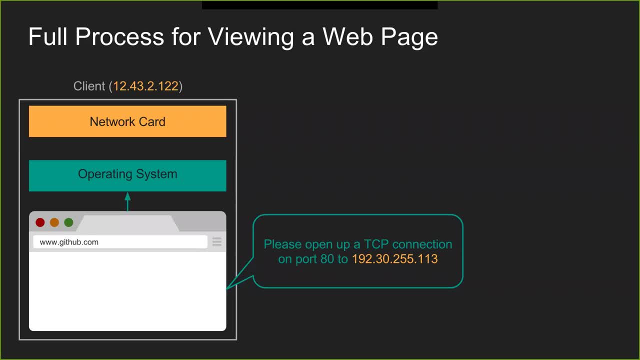 server will then respond: yeah sure. and then the operating system will be like great. the operating system sends a message to the browser being like: we've got a connection established. the operating system, the server, sends a message to the web application saying you have a new connection and they'll pass on to. 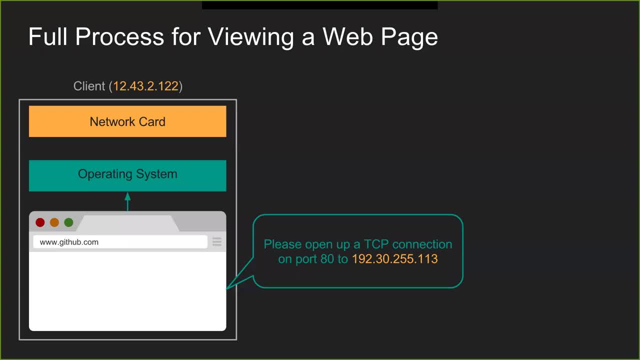 something like express or whatever web server you actually use. this made that like requested from the openness and that it would get this request. then, um, at that point the browser's like: cool, I'm gonna send a request for this web page I want to load. so it sends a request for the web page along with all of the headers, which 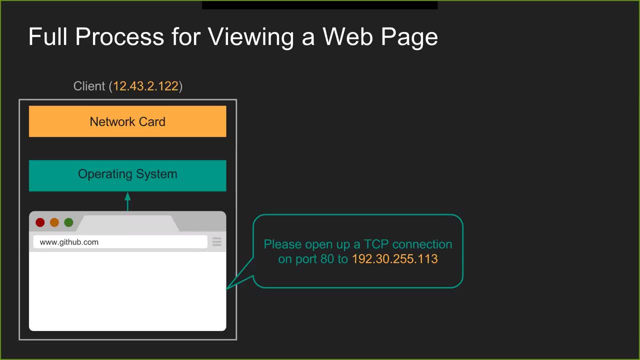 includes cookies and stuff. a web browser, although the website than responds with. this is the web page, the web browser. we're like cool. these are the other files needs. later I'll send ten more requests. now we're the browser will be like cool. here are 10 more files. 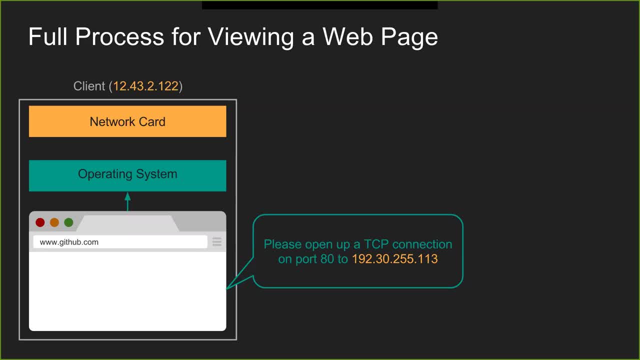 And then the browser will be like: damn, I need to load 20 more files so it'll send 20 more requests. Then eventually, the web browser has everything it needs can render the page and you have a web page. 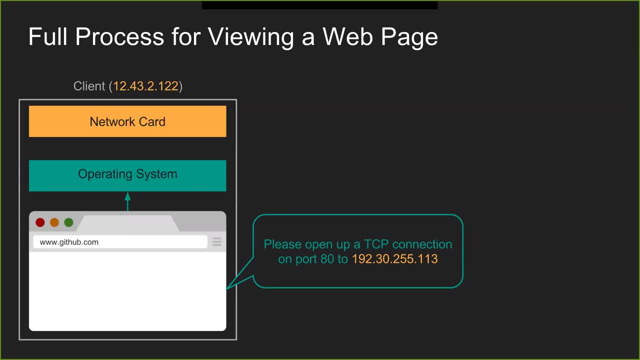 And that happens super quickly, But not always. Sometimes it's really hard to optimize to make sure that, especially if you're connected to a server on the other side of the world, because then you've got a 300, 400 millisecond delay. 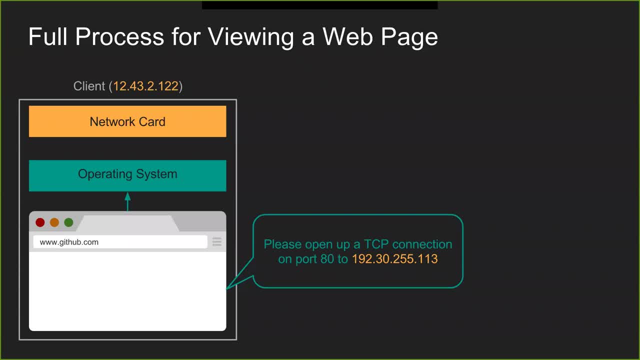 then each round trip takes 400 milliseconds. So if it takes four or five round trips to get everything, that's three, four seconds to load a web page. That's before even rendering it. So this is actually. there's a whole field. 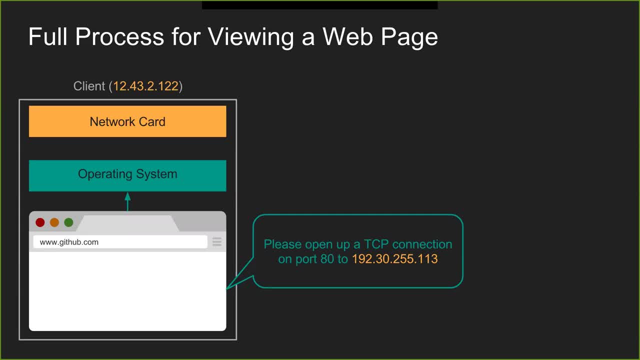 about optimizing this. Facebook actually used machine learning to crazily send various different they're like, they experiment across their billions of users with all these different techniques and they work out using crazy maths which one's probably the best, and they tend towards that to speed up. 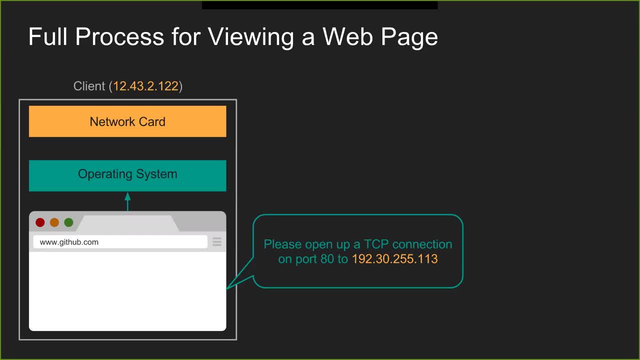 page download and rendering times. So it's like if you can apply ML to it, then it's a crazy field. But there's this whole field about making sure that you optimize and get everything over to the browser as quickly as possible, which is kind of interesting. 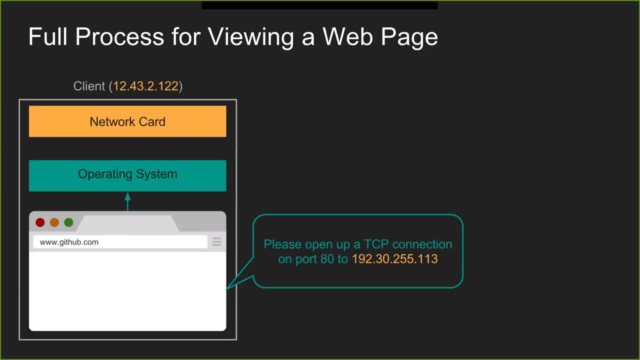 All right, I guess that's all the content I prepared. I wanted to talk about cookies and sessions as well, but that's probably better suited for an interactive code session the next time. Are there any closing questions? Yeah, I just have a random question about. 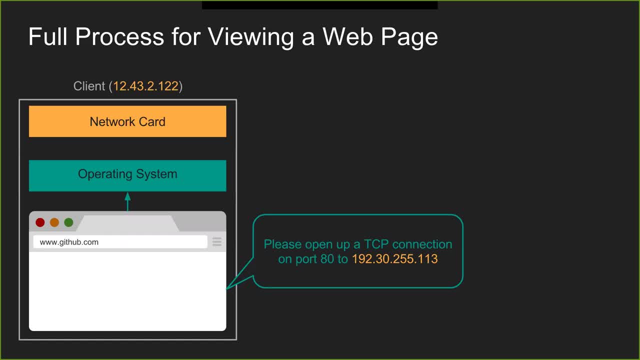 it's interesting to me that there's a separate battery for the clock. Clearly it's really important to keep time because I'm remembering why you picked it. Yeah, Because it's so important to keep time. I imagine there's a lot of programs that depend. 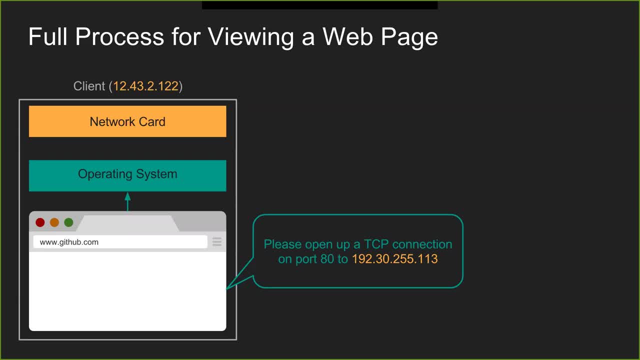 on the time or something. And why was Y2K a thing? I mean, we're so afraid of the time. It seems like all the programs that I use it seems like they would work without the time, Right. So one of the most important uses for time. 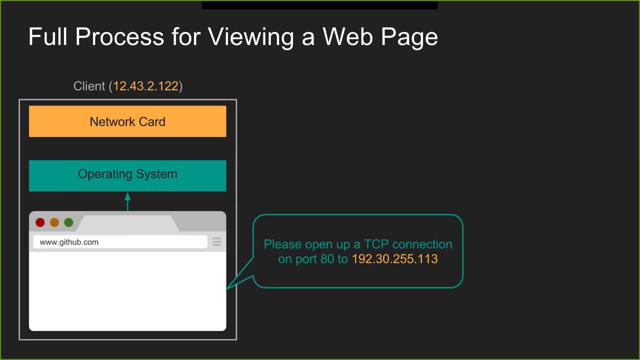 is. sometimes they're used in protocols in exchanging information and stuff, In particular security protocols for establishing secure communication with someone. There's been a trend in the security industry of designing protocols that don't require you to know about time, because it turns out. 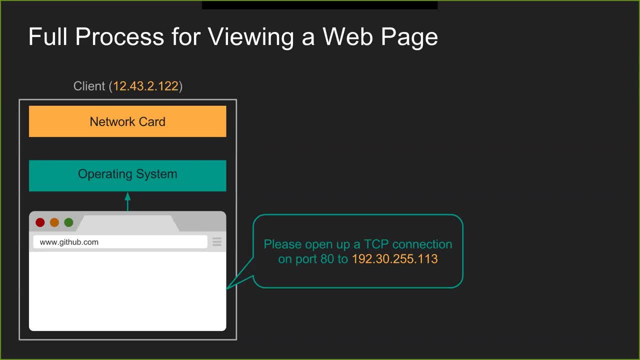 that time is easy to. if you're on the same local network, it might be quite easy to intercept someone's NTP and change the time on their clock and change the time on their computer and then be able to use that to break the encryption. 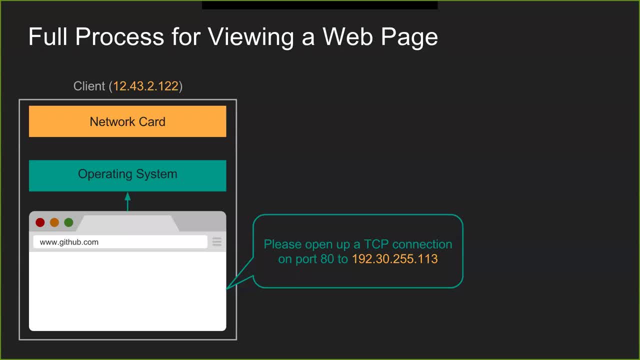 Which is only something that's been done recently. But time is used in protocols is the biggest use case for it. Other than that, anything UI related that relies on the time- lots of stuff If you have protected copyrighted content on your computer or device, say, for example. 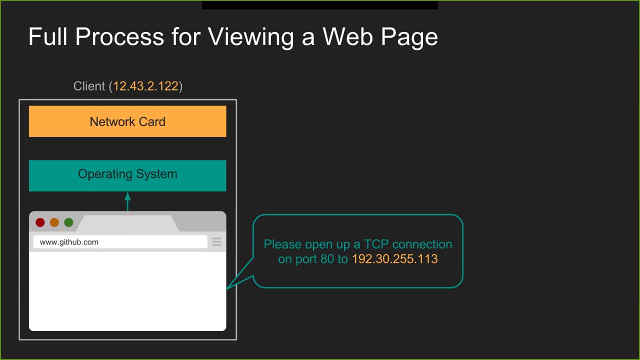 on the PlayStation when you rent a movie or on your computer when you rent a movie, it's important that the time's correct, because otherwise you can watch it for longer than you're allowed to If you have software that uses licenses that expire after a certain amount of time. 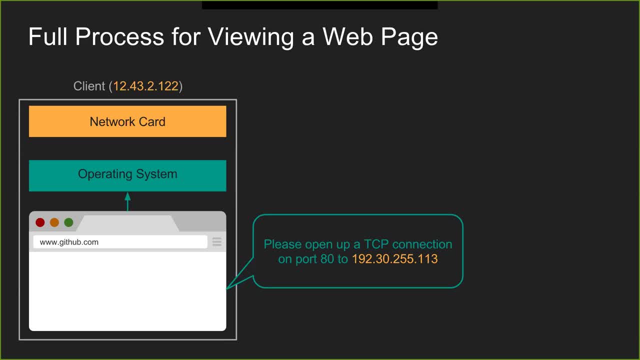 they use the clock. A common trick to get around, that is, by changing your clock, Which I may or may not have done in the past- Sounds like other people here may or may not have done in the past. I do not condone or whatever. 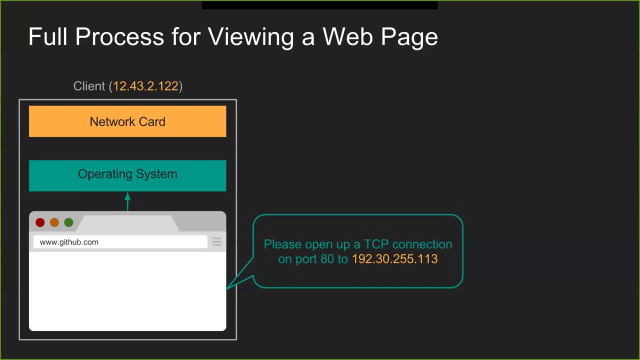 But it totally works. Yeah, so time is used for lots of things. Yeah, any other questions? I have a question? All right, I'll stick around for a little bit. Feel free to come ask me more specific things. I can go into super detail about anything on here. 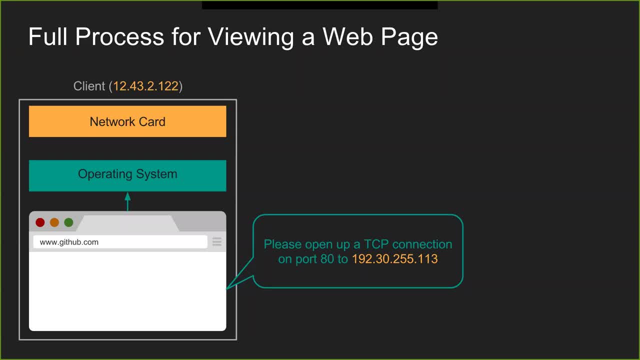 or clarify anything or explain something in a different way if it wasn't clear. Yeah, Yeah, Yeah, thanks for having me. It was fun, Thank you. Thank you. Why did I not have any cat pictures?